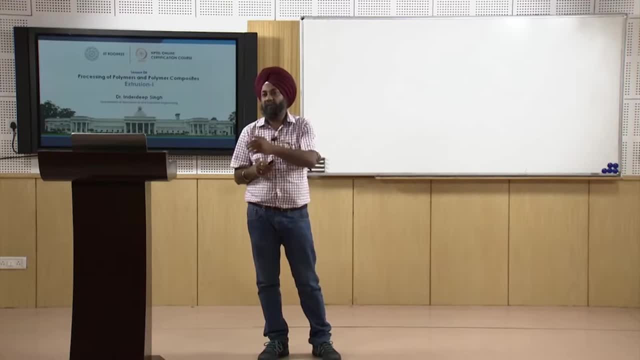 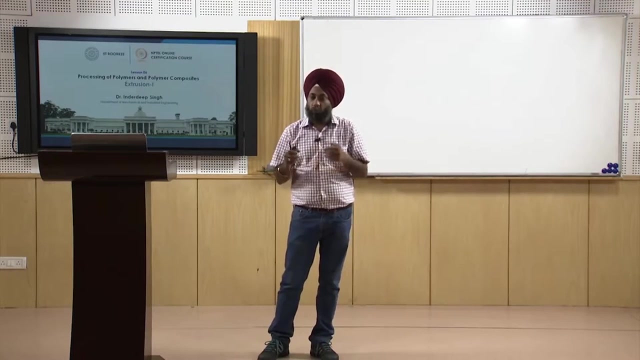 both the processes, plus in the processes that we are going to cover in our subsequent lecture. you will try, you will understand that there are three components- again i am emphasizing that- heating, forming and cooling- that are common, so that we are going to see today. also, if you see the topic that we are going to cover today, it is extrusion, now extrusion. 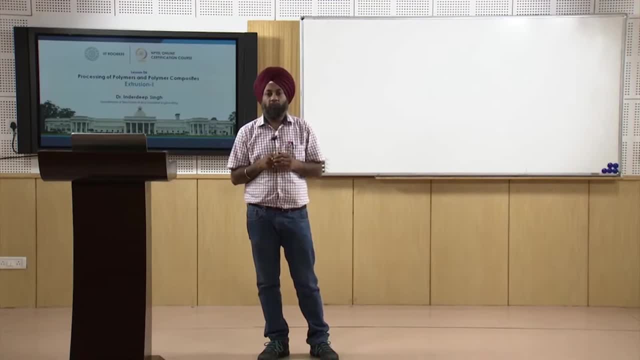 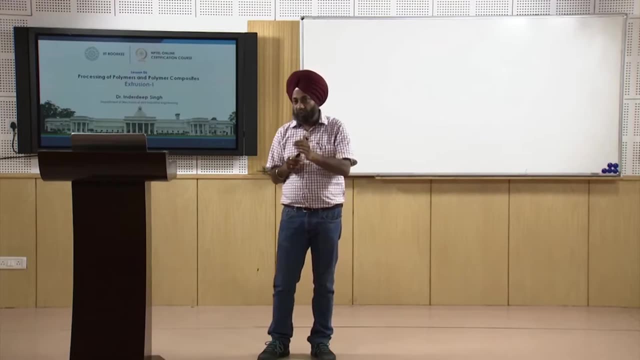 is a most widely used process for processing of polymers and we will see ah that how the plastics are processed using extrusion. what is the process? what are the various parts of extrusion machine? we will try to understand that. what are the important control parameters? what are the different types of products that can be made? 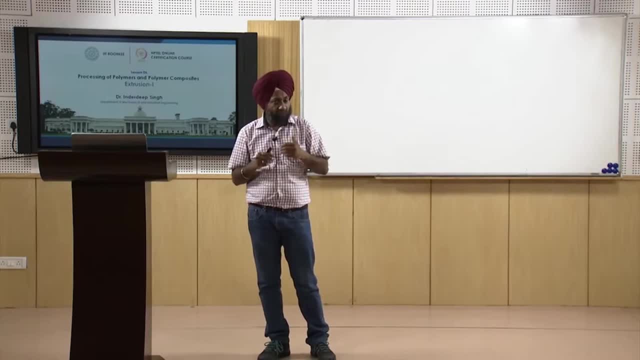 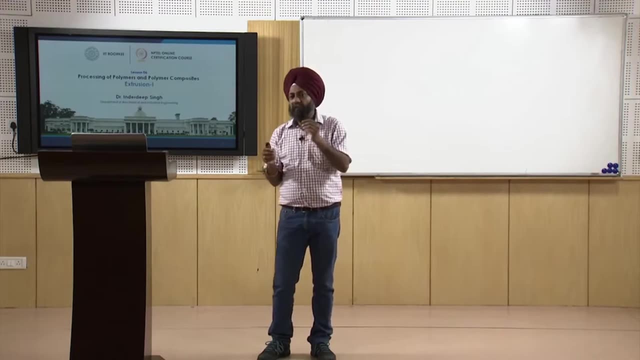 and then we can always ah understand the things better if we have a video which represents the process. so today we will see a very small video which represent all processes. so exactly any process is different, so that we will try. we can always seen the process using this. 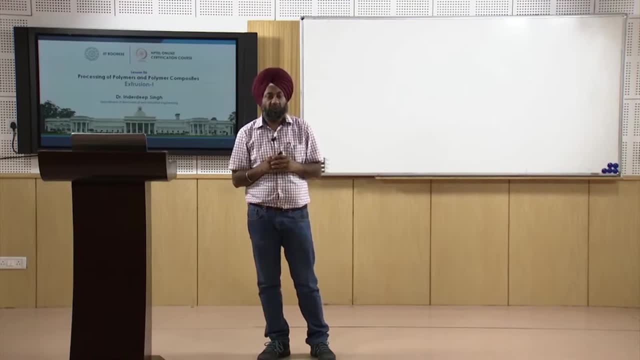 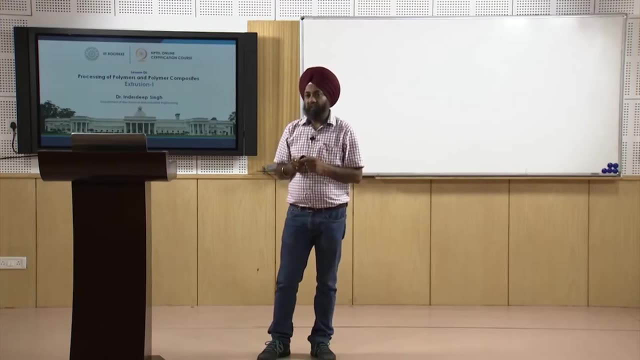 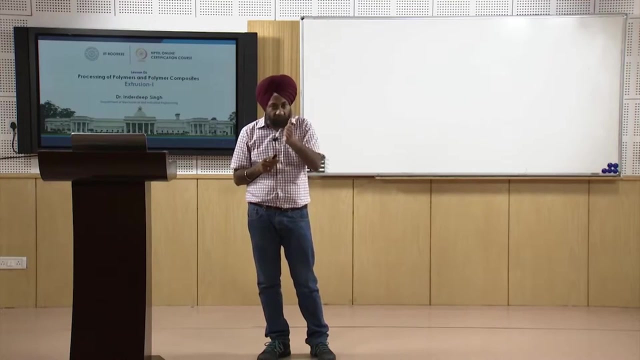 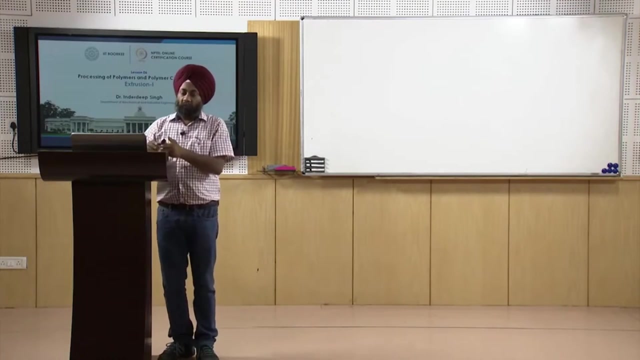 will give a complete description of the whole process, that how the process operates and finally makes a product out of a plastic. so let us start our discussion on extrusion and we will cover whatever i have listed down in the beginning of the session, that all these things will be covered in todays session. so let us start our discussion. 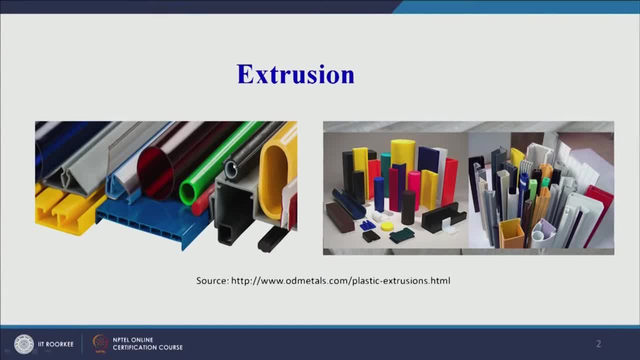 on your screen you can see the different types of products with different colors are processed for plastics. so if you see yellow color, blue color- and first let us start first- i want to grab your attention towards the products that are made. then we will go to the technical. 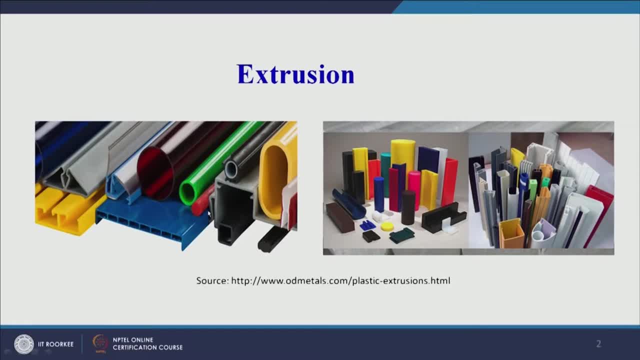 aspects of the products. if you see different colors, products can be made. that is one versatility of the process, that it is not color specific. any color can be made. so if you can appreciate that, then you can see the shapes, which is a technical parameter. so if you see the shapes, 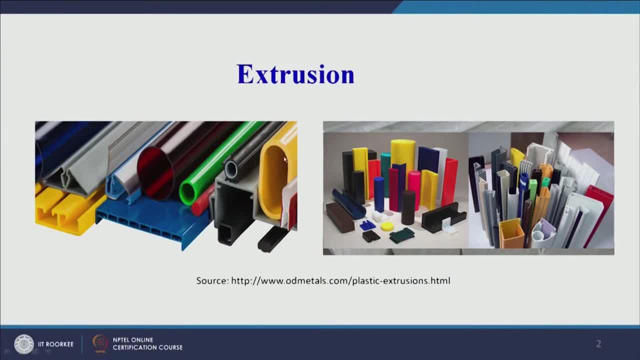 there are circular cross sections. there are maybe, ah, different types of cross sections. square cross sections are there, oval type of cross section is there. then we can see, ah, special design, a honeycomb type of cross section is there. so, depending upon the cross section, we can make a use of the extrusion process and we can make a product. so, on this, 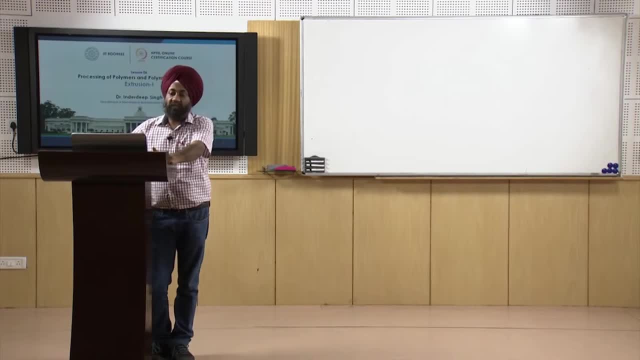 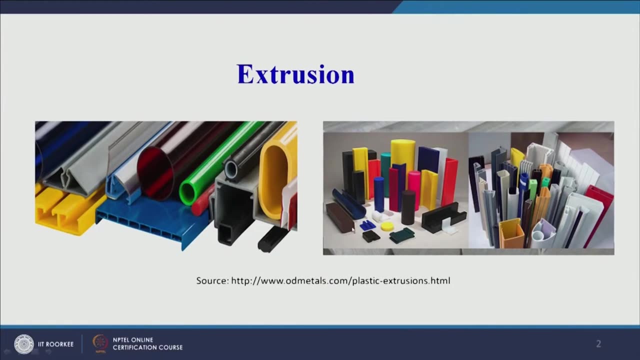 side, also the other view of these products. you can see there is a angle section here. there is a solid cylindrical cross section. the solid cylinder has been made. there is a rectangular type of cross section and there is a complicated cross section also. so extrusion process is a versatile process. 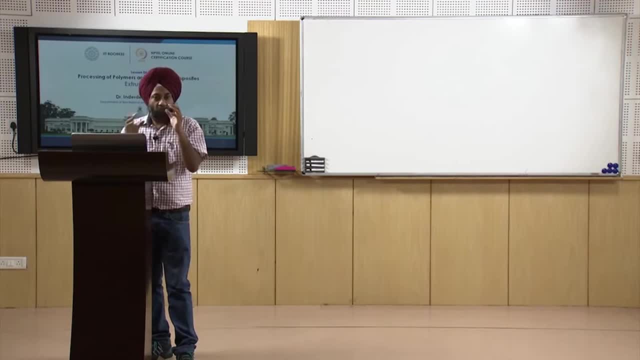 and everything depends upon the die, or the or the hurt of the extrusion machine, that is, the die. now, depending upon the product, we have to design the die, and the die will give us the desired shape. the things, as i have already told, we have to heat the plastic. 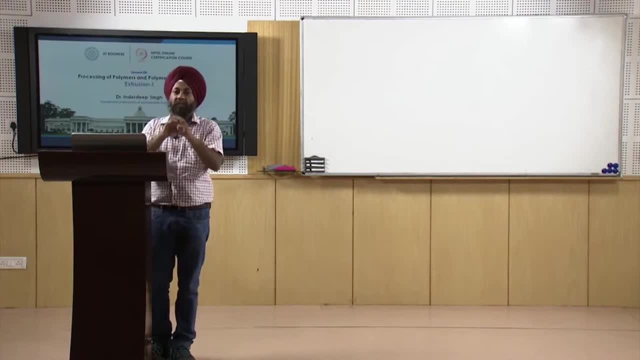 material. once it is hot, it will be pushed through the die. depending upon the shape of the die, it will take the desired shape. finally, the product that is coming out of the die, we will cool that product and finally, our product will be ready and, depending upon the 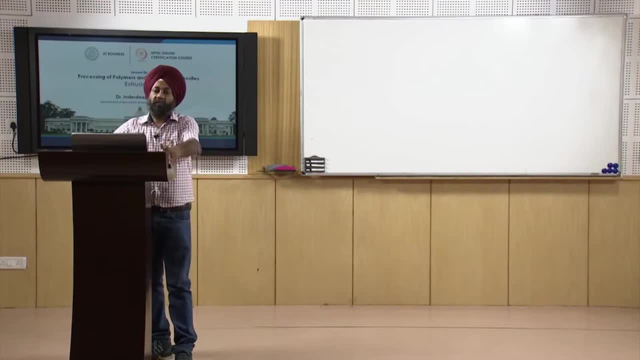 length that we require. we will cut the product into desired cross sections or not the desired cross section. So we will cut the product into desired length across the cross section so that we get the product. in the video it will be very, very clear so you can see the different types of. 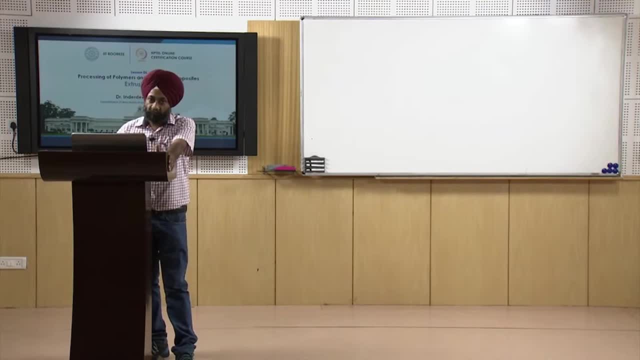 products that we can make using the extrusion process. just to explain you the importance of this process, i can just share with you that: the gardeners pipe that we use in for watering the plants or sometimes for washing our cars. also the plastic pipe that we use. 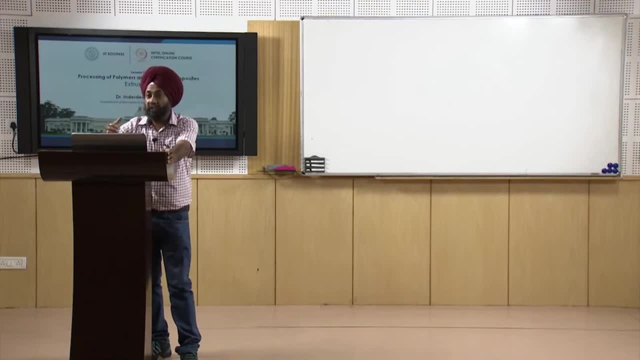 that is made by the extrusion process, So that you can appreciate, relate to the process. So let us start our discussion with extrusion process. extrusion is a high volume manufacturing process, so you can see it is a continuous process. once you feed your raw material, which 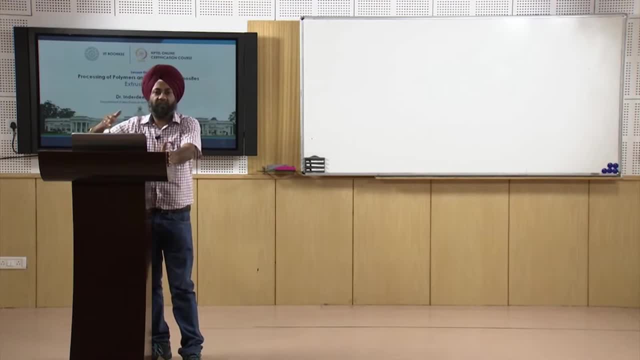 is available in the form of pellets. so these pellets will be melted and then they will be forced through the die and continuously the production can be there. so if you see you have long gardeners pipe, long hose pipes, so that that means that they have been produced. 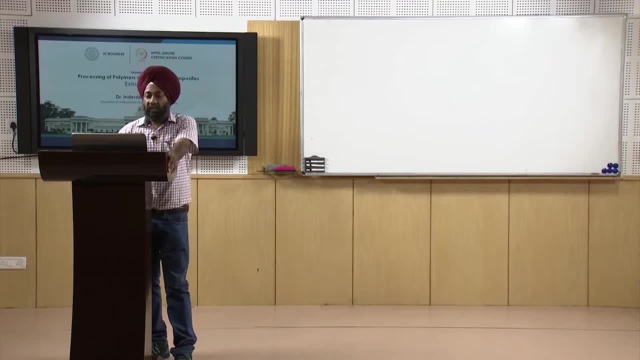 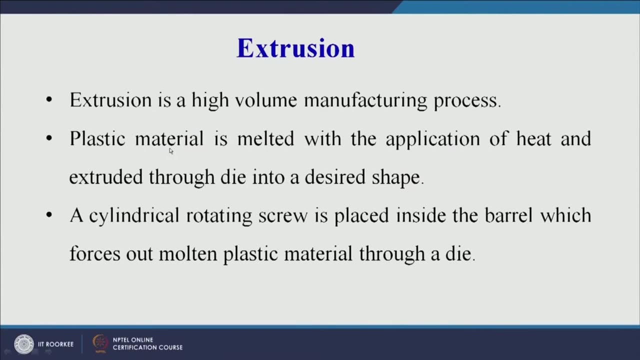 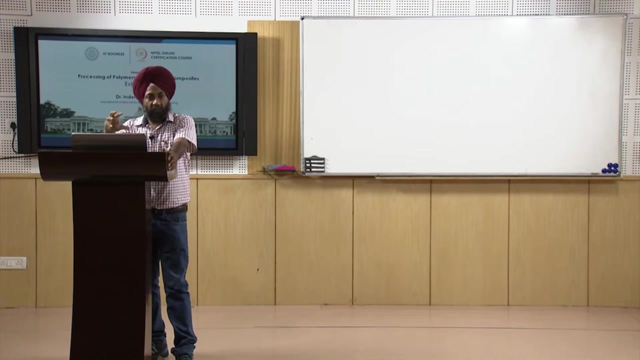 through a Continuous process of manufacturing. so extrusion is a high volume, continuous manufacturing process. plastic material is melted with the application of heat and extruded through the die into the desired shape. i have already emphasize this point: that heat for your heat, your deformation, ah, in the form of a die- and finally the cooling are the basic principle. 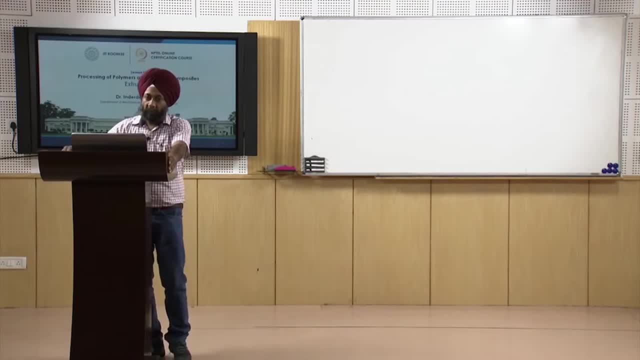 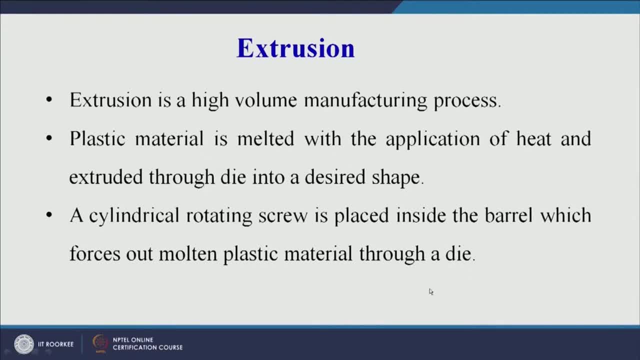 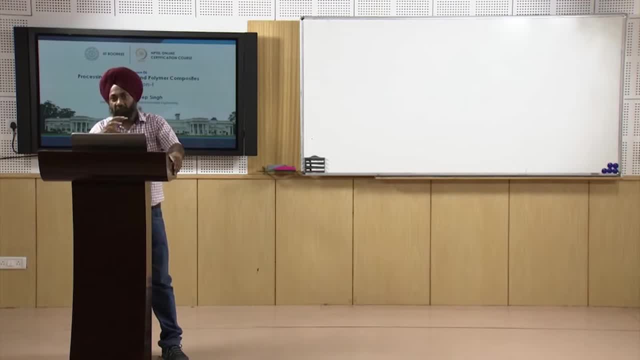 A cylindrical rotating screw, A cylindrical rotating screw A. digo другой fibula also sudden test whether it is rare or kind of eat. this is impressive. byION is prioritized for such a type of plastic material. second step: Start gosh is very important. that is hi join by, joining in this kind of plant habitat. 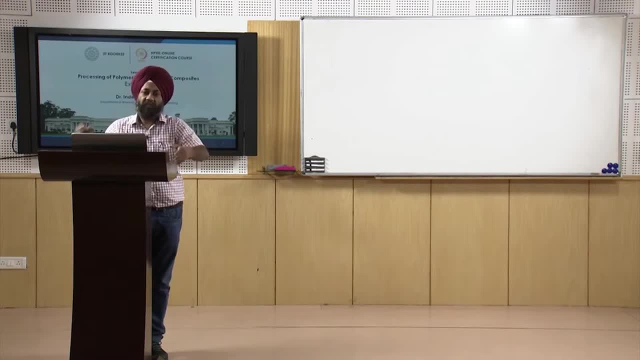 worldwide是不是 timingِّ suffer? i 말 interq, do not. then things are, by the pressure we can bring Does Of Inside Through The 20 warenman thanks you To. In All right, ALEXANDER, ONE LINE REFER, snuck up in for is one half or those whoرا we no longer share. 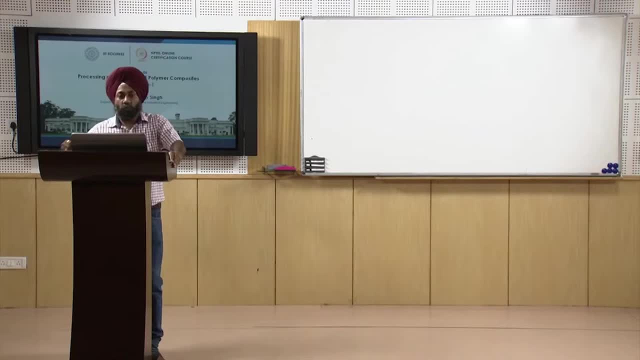 he put into the human body or into the animals body. so the same principle, you can correlate that medicine with the plastic. now you have a plastic inside a barrel. you have to push it so that it comes out. so dike in this case can be the needle through which the medicine comes out. 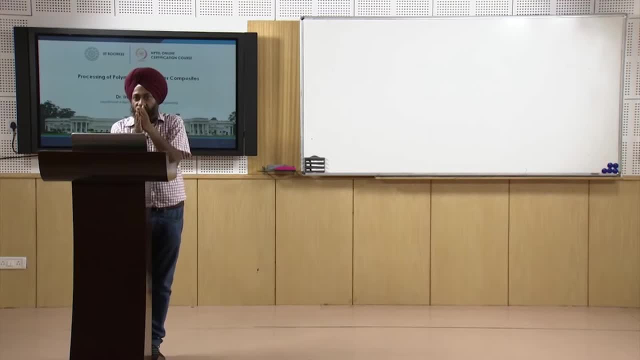 so that is the principle, but here that piston cylinder arrangement. in place of the piston cylinder arrangement, many a times we use a screw and barrel arrangement through which we have the plastic. we push that plastic with the help of a screw and it is forced through the die into the mold cavity. in this case it will not be a mold cavity, it will be a 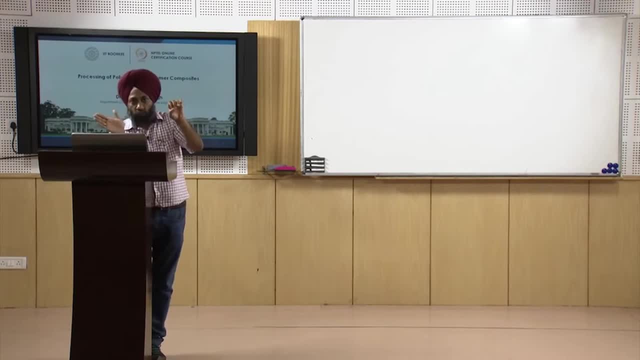 die. so you will push the molten plastic through the die, and die will be the exact replica of the final product that we want to make now. as i have shown in the previous slide, different types of products can be made. on your screen you can see. so these products. 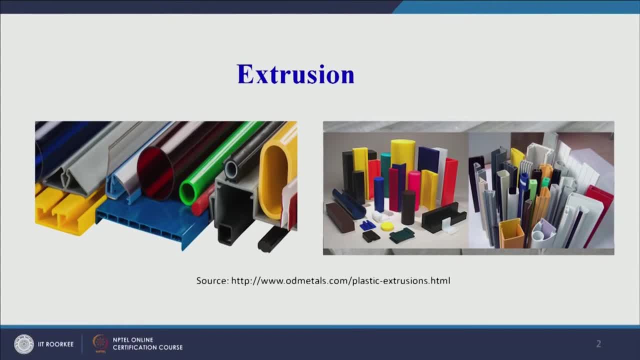 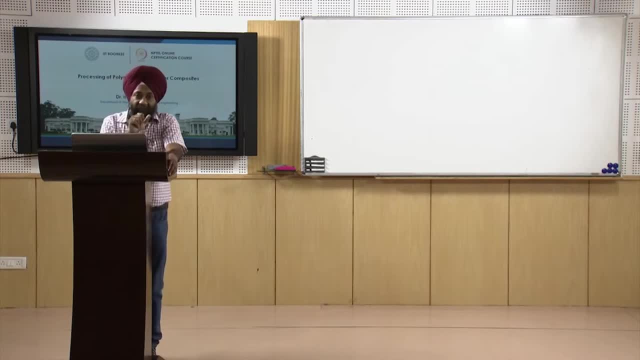 the shape of this product will depend upon. you can very easily now answer this question. the shape of this product will depend upon the shape of your die. now, if it is a circular die, you will get a circular product. if you have a square die, you will get a square product. now, depending upon the 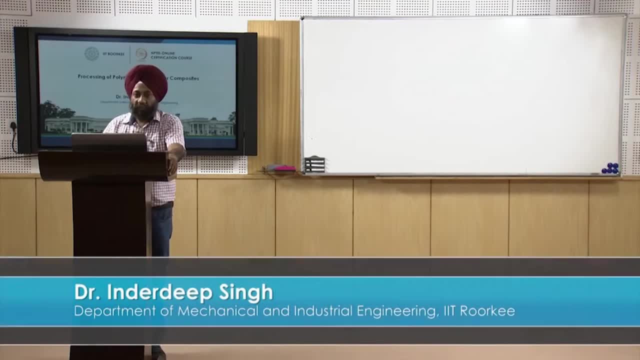 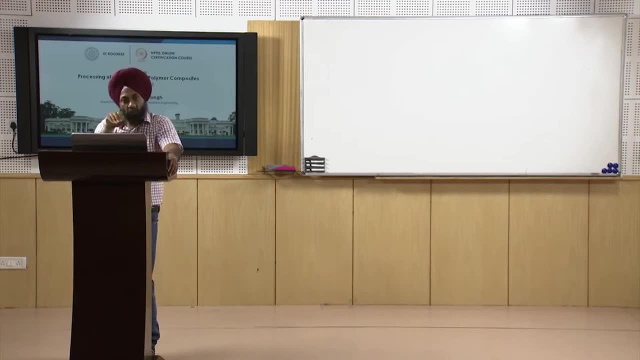 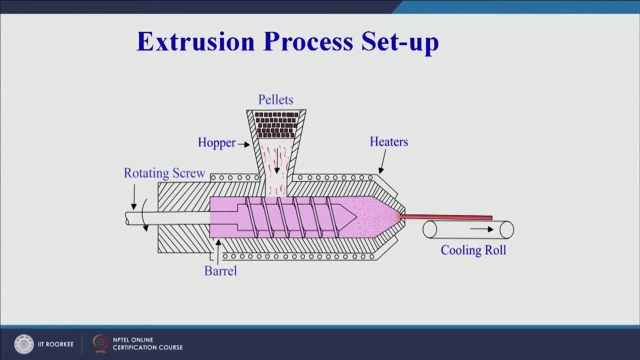 shape of the die, you will get your product. so that is, this is the. these are three basic steps, that is, heating of the plastic, pushing of the plastic through the die and cooling of the product when it comes out of the die. on your screen now you can see a very simplistic representation of the extrusion process there. 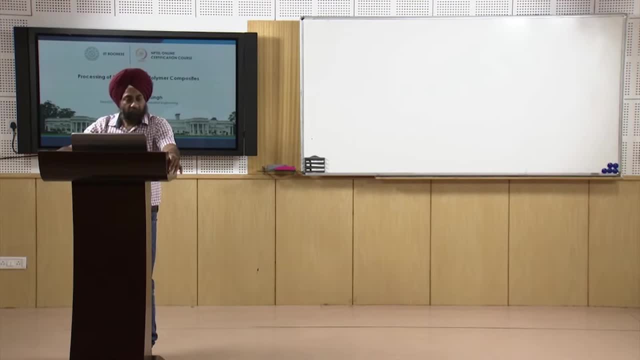 can be so many other components in the extrusion machine, but we are trying to understand the very basic mechanism of the extrusion process. so if you here, you can see there are for any process. there are three things the those are important. first is the raw material. second, 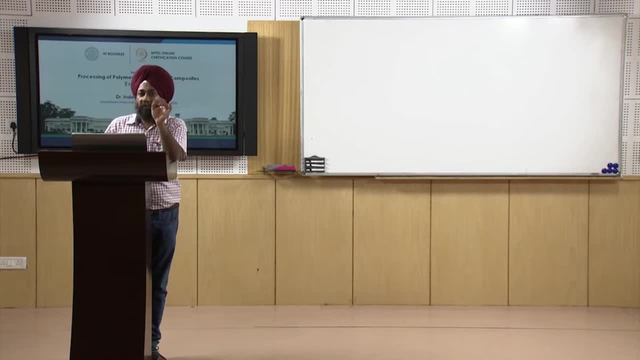 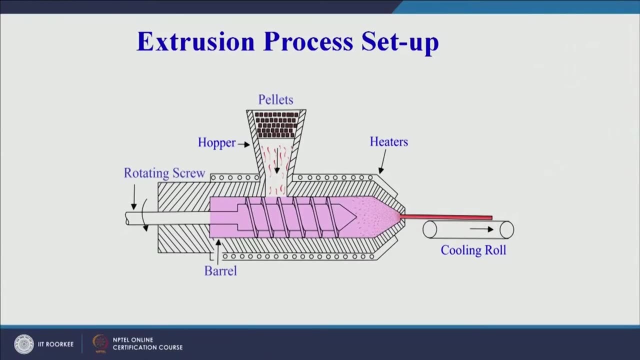 is the process mechanism and third is the product. so here let us start from the raw material. so raw material, in case of for extrusion process, are the pellets on your screen. we have this setup. these are black portion particles. are the pellets. so usually we get for thermoplastics we get spherical pellets, and those pellets 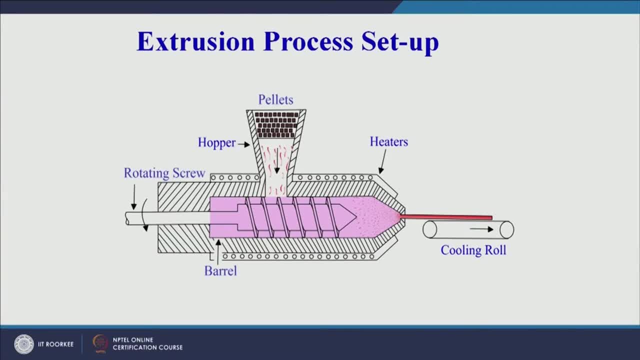 act as the raw material for the process. this, these pellets, move through this hopper into the barrel. this is the barrel portion. i am highlighting that barrel portion. so that is the barrel, and there we have this rotating screw. the rotating screw has also a specific design that we will cover towards the end of today's session. so there is a screw. 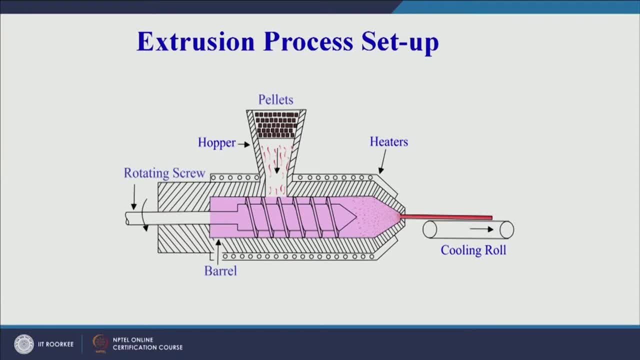 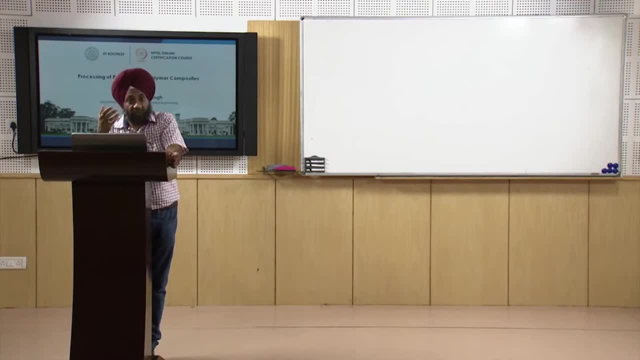 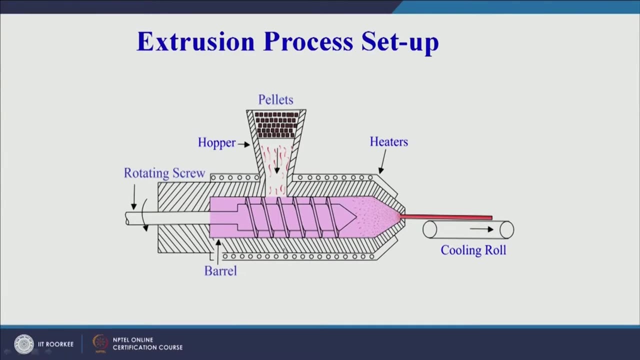 there is a barrel, there are pellets that are coming down. now pellets are solid, spherical particles. now we have to melt them, and for melting we require heat, and for heating we require heaters. so on your screen you can see all around the the periphery of the barrel. we have heating arrangement. 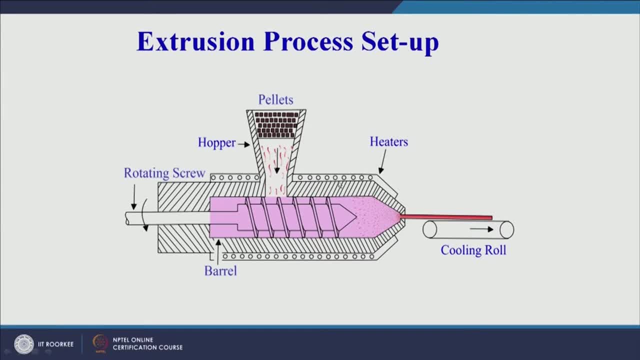 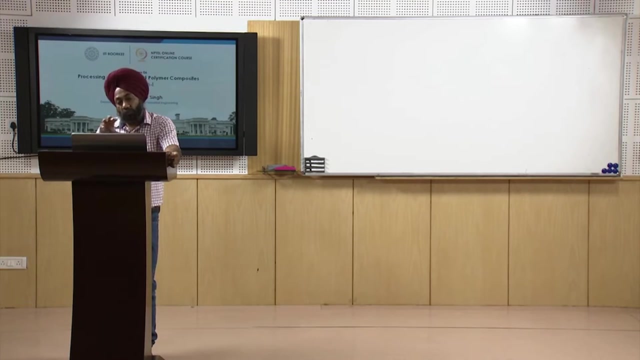 These square dots- sorry, these circular dots- represent the heaters. so these are the coils, or the heating coils. these circular coils here also represent the heaters. So you have heaters all around the barrel. So these heaters will heat the polymer pellets and will melt them. and once you melt them, 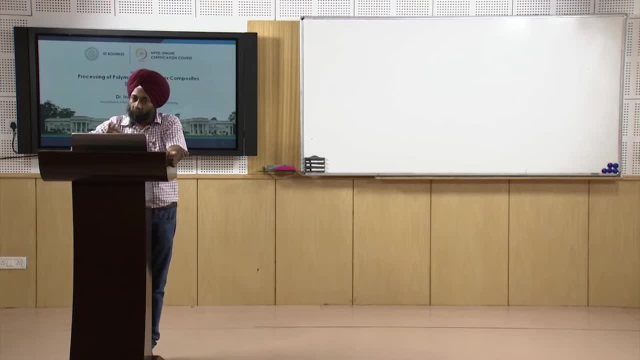 next stage is you have to push them through the dye and then your product will be formed. So here we have the dye arrangement, This is the place where we will have the dye, and then this red color portion is the final product that is coming out. 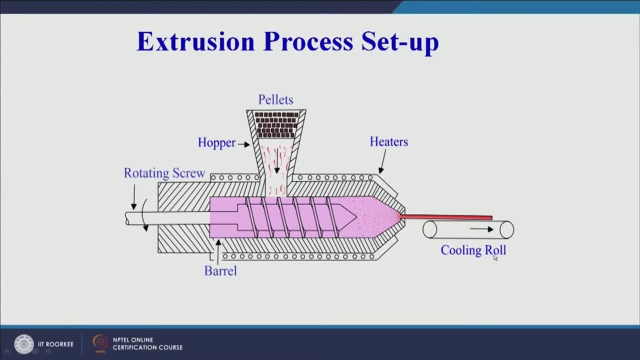 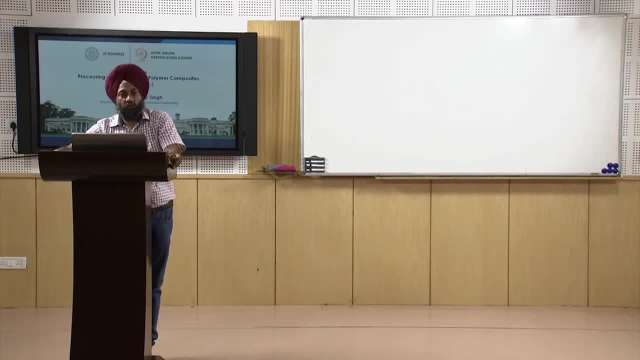 Now this product is rolling on a cooling roll and we can have. we will see in our subsequent slides when we will try to study step by step that how the process operates. We will see that the cooling can be water cooling, It can be air cooling, but right now, with the help of this diagram, we are trying to 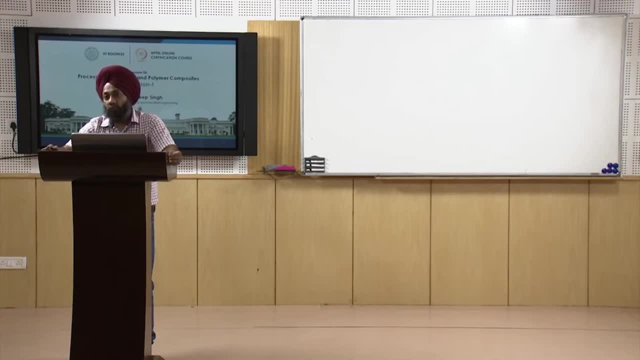 understand the how the extrusion process works in case of plastics. All of you may have studied extrusion of metals, So there are different variants of extrusion of metals. but here, in case of plastics, there is slight modification as compared to how the raw material is fed into the machine. 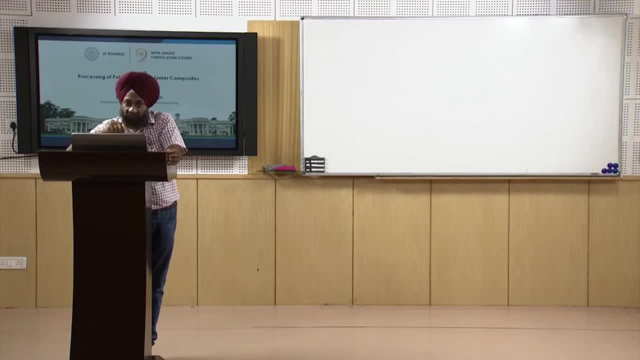 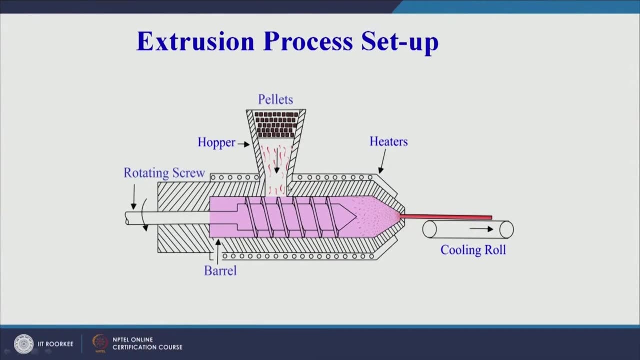 how the product comes out from the setup. All these are the different things Compared to the extrusion of metals. So here you can see once again- I am repeating just maybe 3 or 4 sentences- We have polymer pellets, thermoplastic pellets. here 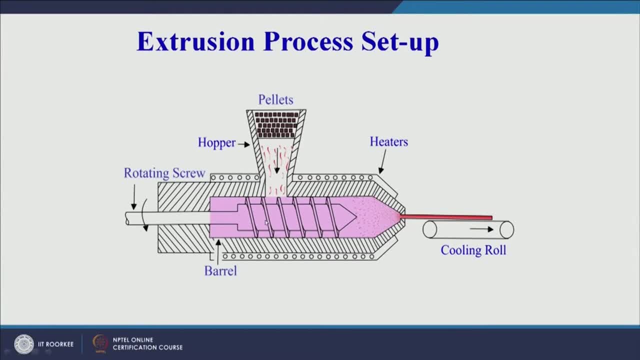 These pellets are fed into the barrel. There is a rotating screw inside the barrel. The barrel is heated with the help of heaters. all around the periphery of the barrel. The rotating screw rotates and it pushes the molten plastic through the dye onto the cooling. 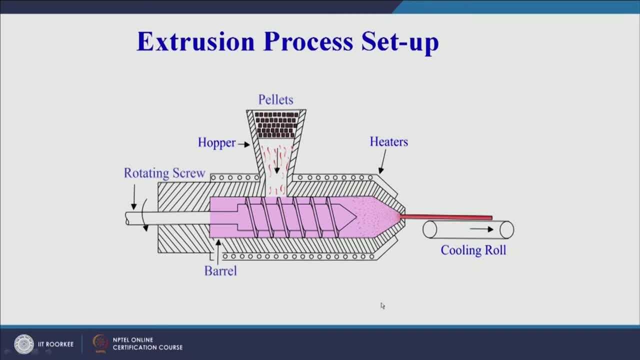 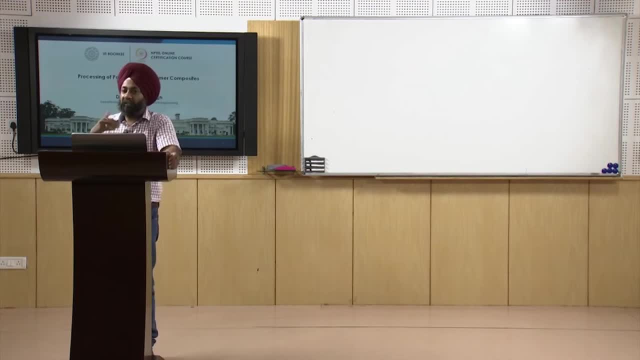 roll and your final product comes out from the dye. So that is the basic working principle of the extrusion process. Now let us read whatever I have said, so that we are able to remember that what is extrusion process actually? Now, plastic material in the form of pellets or granules is gravity fed from a top mounted. 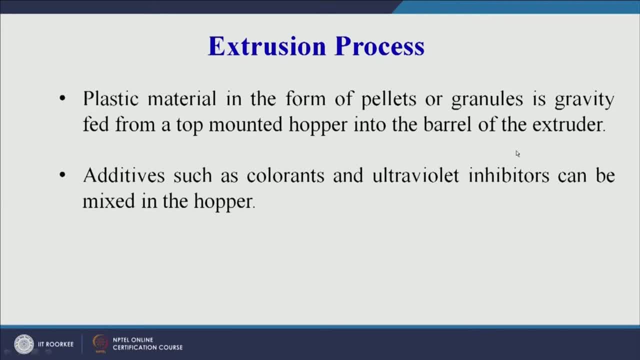 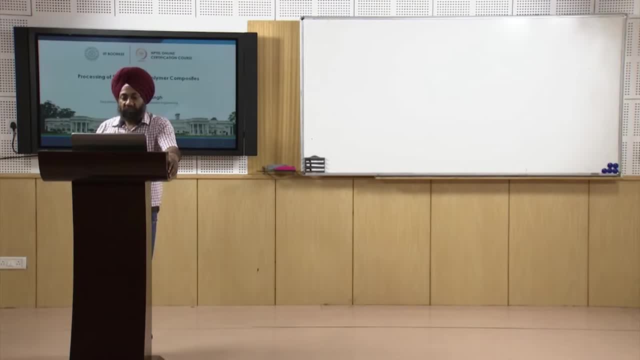 hopper into the barrel of the extruder. I have already explained. the raw material is in a hopper. It is gravity fed means it comes down by its own weight. Additives Such as colorants and ultraviolet inhibitors can be mixed in the hopper. 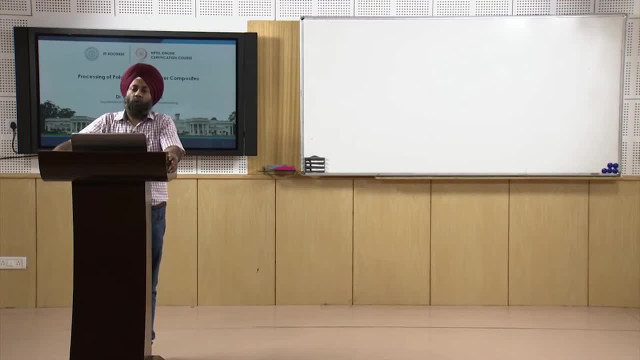 Now this is important. you have seen so many different colors of products were there in the very first slide There was yellow color, green color, black color. So these coloring agents we have to add in the hopper. We have to prepare a batch of the raw material which will have the pellets. 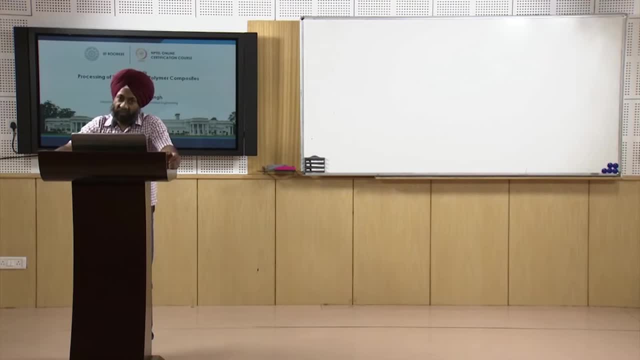 Other additives, sometimes fire retardants, may also be added at the raw material mixing stage only. So here coloring agent will be added. Similarly, ultraviolet inhibitors can be mixed in the hopper. Now ultraviolet inhibitor. many a time we see decoloration of the plastic products takes. 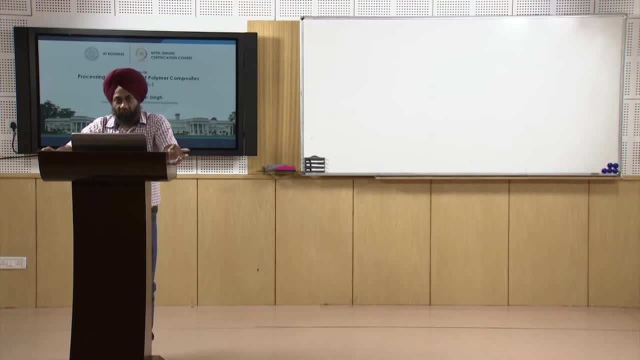 place. if suppose the bucket lies in the sunlight every day and for months, all together, for years all together, the decoloration takes place. So we can add some inhibitors which inhibits the decoloration of the plastic parts. So all those things, raw materials, can be added in the hopper. 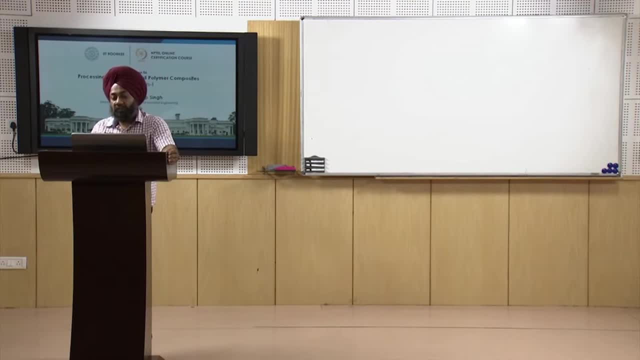 5. Plastic materials. Plastic materials enters through the feed throat and comes into contact with the rotating screw. Now feed throat is at the end of the hopper. So you have a hopper, there is a feed throat at the end and through that the raw material. 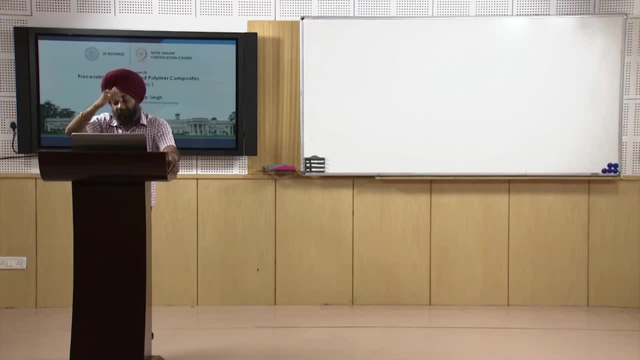 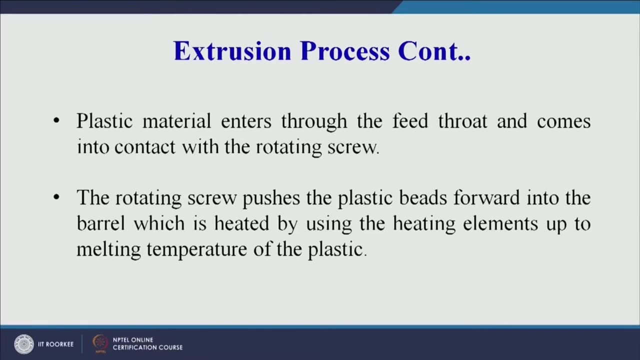 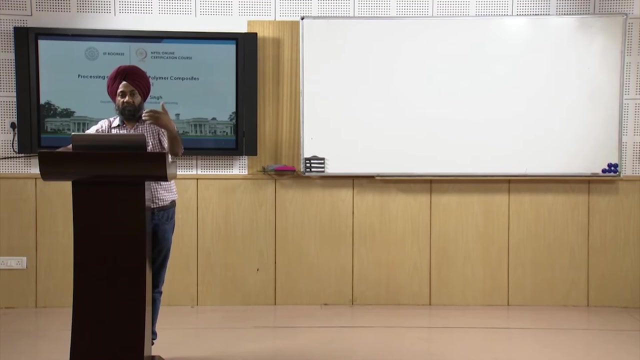 in the form of pellets and other additives adds, enters into the barrel. The rotating screw pushes the plastic beads or plastic pellets forward into the barrel, which is heated by using the heating elements up to the melting temperature of the plastic 6. We will melt the plastic because of the heating arrangement that we have provided around the. 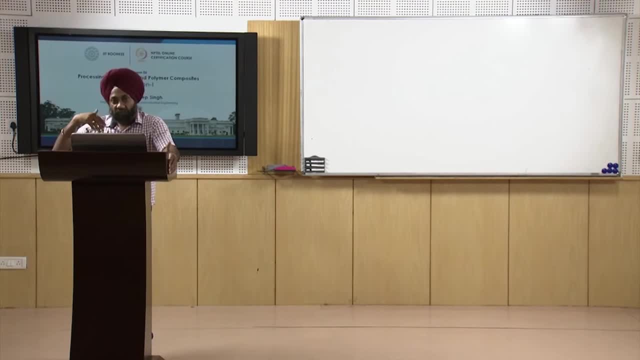 barrel. So once the plastic is in the molten state, it will start to flow, and then we will push this molten plastic with the help of a rotating screw through the die. So the next stage is the plastic material is completely melted in the melting zone. 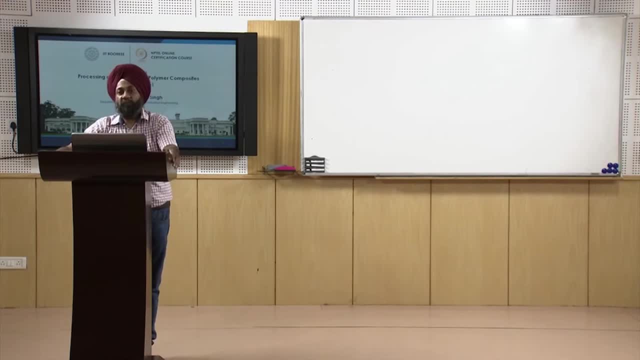 So we will see the design of the screw and there are 3 zones specifically for specific task that we will see later. 7. So the plastic material completely melts in the melting zone. 8. The thermostat is used to maintain the inside temperature of the barrel because we need 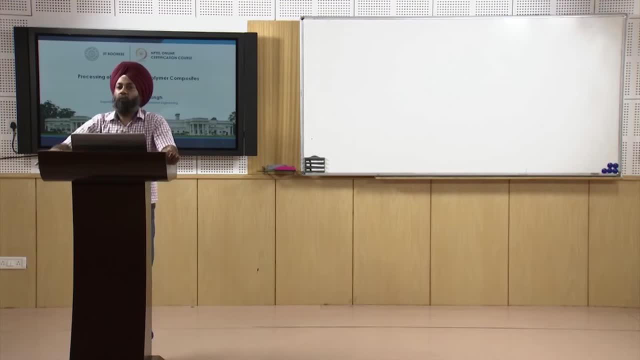 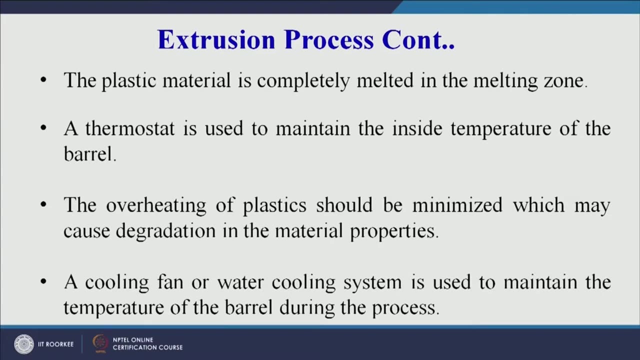 to maintain that temperature by the time we push our molten plastic through the die 9.. The overheating of plastics must be minimized, which may cause degradation of the material properties. Now we have to see that how much temperature we should give to the plastic overheating. 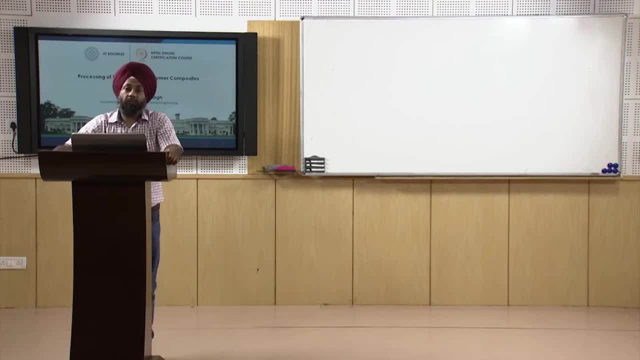 of the plastic is also not is also not advisable. why? because it will degrade the properties of the product. So we have to be judicious in the choice of the temperature that we are going to give to the heating elements, So that we are able to control the properties of the final product. 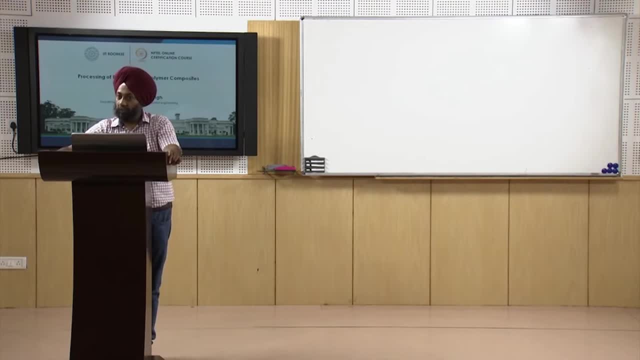 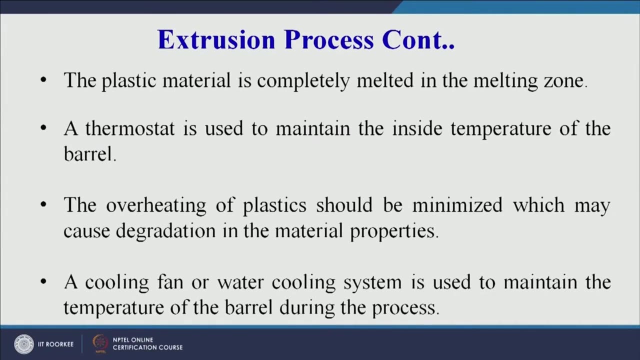 So the overheating of plastics has to be avoided. we should always keep this thing in mind. 10. A cooling fan or a water cooling system is used to maintain the temperature of the barrel during the process. So this is an another important point that we need to maintain the temperature in the 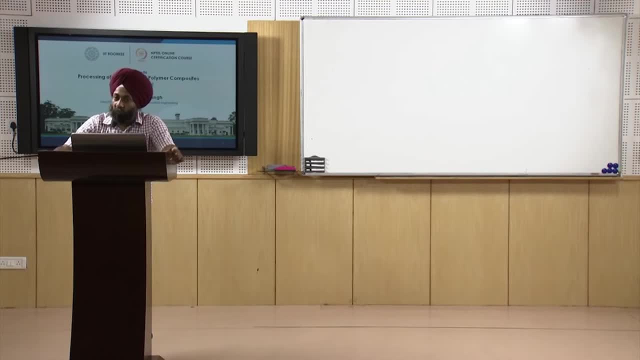 barrel. for that we have heating elements. 11. To avoid the overheating, we have the cooling arrangement, that is, the fan, or a cooling system is provided. 12. Now there are other arrangements. as I have told you, the diagram that was shown is a very 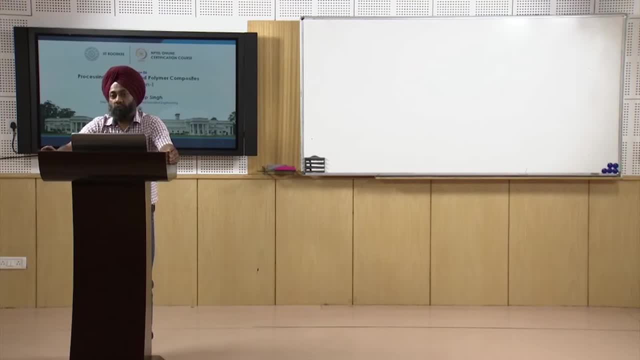 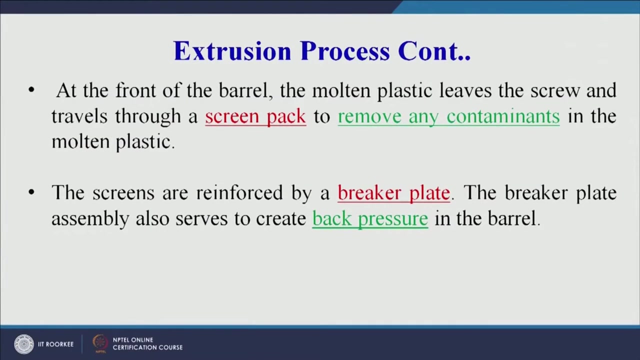 simplistic way to explain that how explosion process actually works. But there are other arrangements also for specific tasks, So we have seen that over. for avoiding the overheating, we have to provide the cooling system. 13. In the case of the barrel, the molten plastic leaves the screw and travels through a screen. 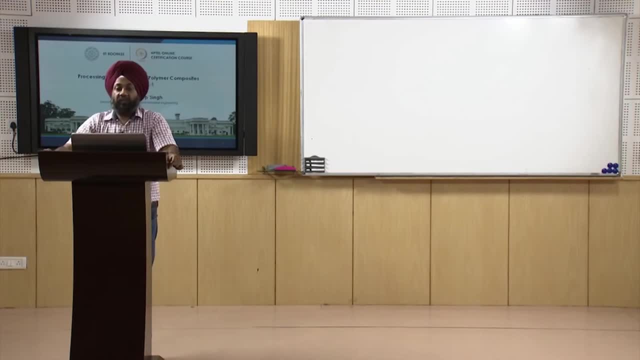 pack. Now what is the role of this screen pack? The role of screen pack is to remove any contaminants in the molten plastic. Many a times we are using the plastic pellets. there may be some undue particles or non-wanted particles all mixed with the pellets, that may travel through the barrel, through the 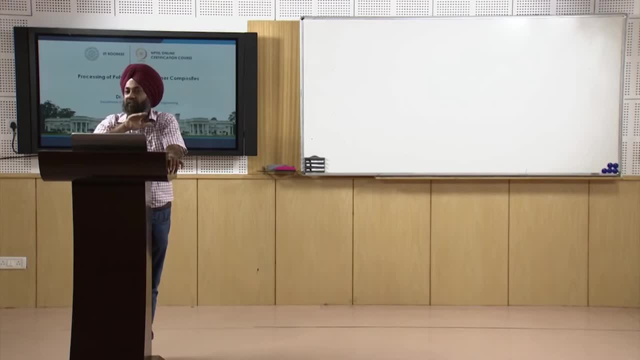 screw. they may be fed through the die. So we need to check that these particles. They may be sometimes causing harm to the die. also, as I have told you, die is the most complicated part of the whole system and the shape, size, surface finish of the product depends. 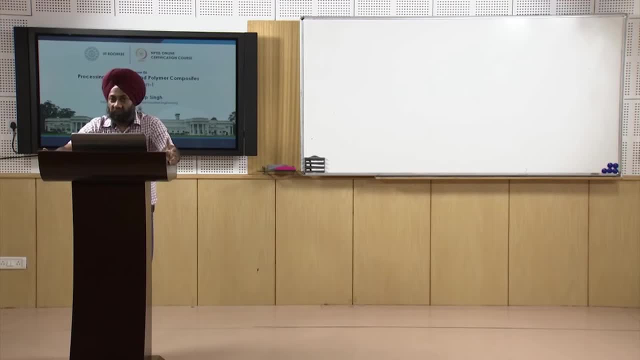 upon the die. So if your die wears out very fast, that is the most costly component in the whole setup. So therefore we do not want any additional or any undue particle going into the die. that has to be avoided, and for avoiding that we can put a screen pack. 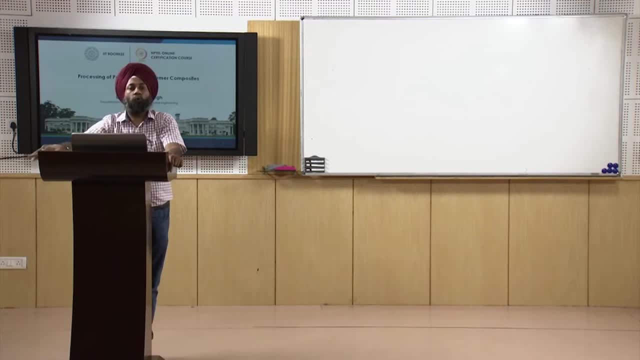 14. Which will only allow the plastic to go through into the die and will arrest all other particles which are not required, or unwanted particles, or unwanted impurities. So the role of the screen pack is to remove any contaminants in the molten plastic. 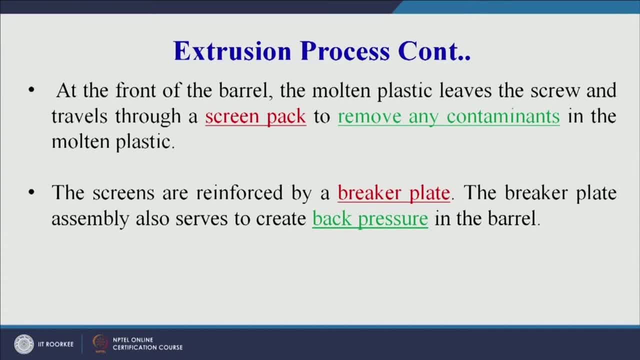 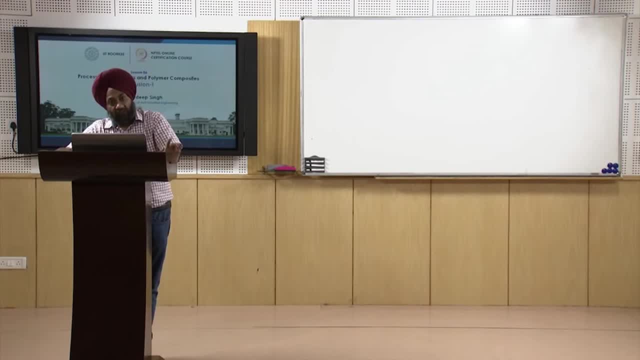 The screens are reinforced by breaker plate. Now, what is the role of the breaker plate? The breaker plate assembly also serves to create back pressure in the barrel. Now back pressure. why back pressure is required? there are two, three terms that have come come up on this screen. 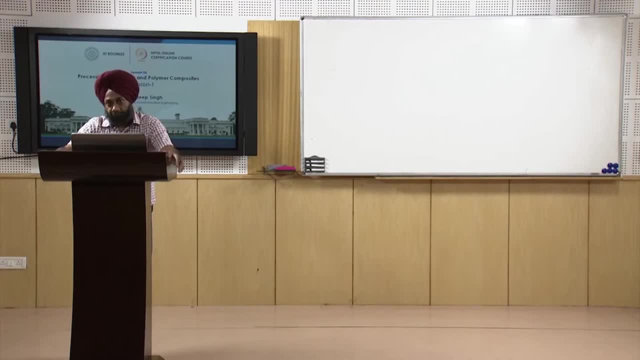 One is screen pack. that is to avoid the flow of the undue or unwanted particles or impurities. with the molten plastic it will arrest those. Secondly, the breaker plate. now breaker plate will apply. also help us in applying the back pressure. Now, what is back pressure? we will see why back pressure is required. 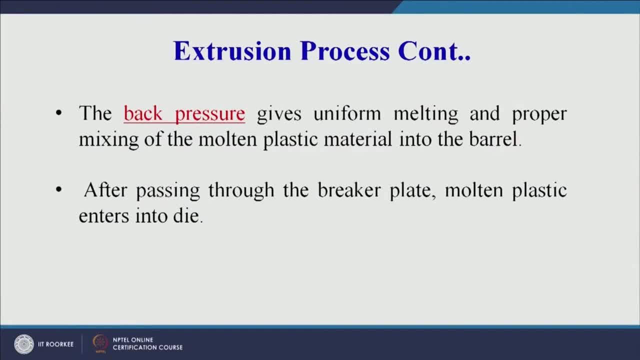 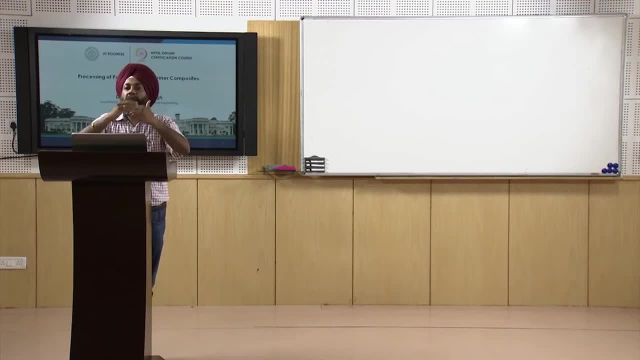 The back pressure gives uniform melting and proper mixing of the molten plastic in the barrel, So that back pressure has to be maintained. 15. So that we are able to properly mix the plastic, the all the pallets melt and there is proper mix mixing, as we- as I have already told that we may be adding some additional, we can say: 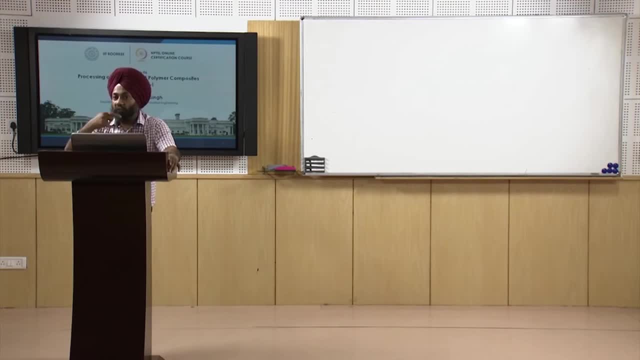 additives in the hopper. So proper mixing is one of the purposes of the barrel, then it is supported by the back pressure as well, as the uniform mixing is one thing and uniform melting is the other thing, So both are mixing and melting. So back pressure helps us to achieve these two M's. the two M's are mixing and melting. 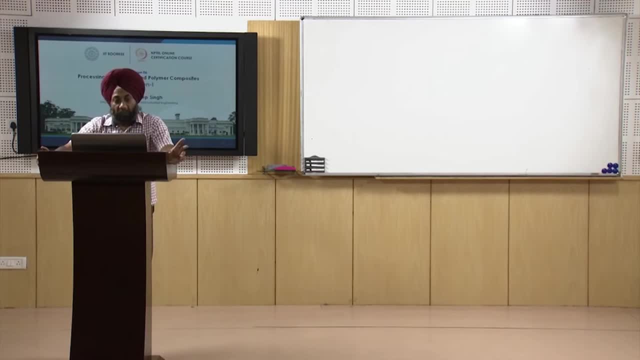 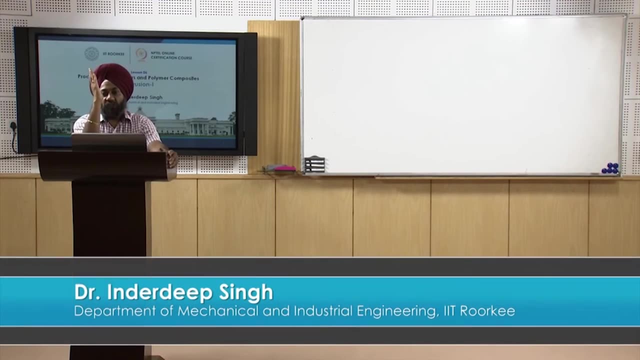 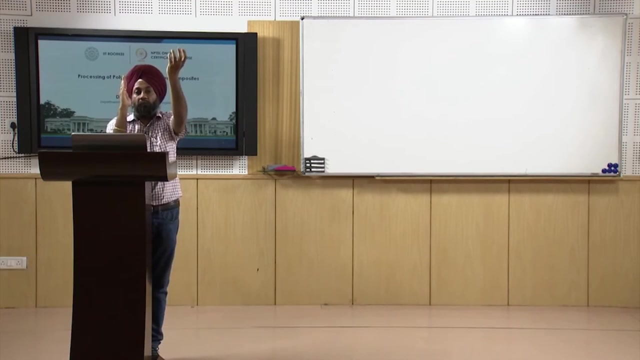 uniform melting and proper mixing. After passing through the breaker plate, the molten plastic enters into the die. Now die is, we can say, is one stage. die is one stage. before that, what has happened? the molten- sorry, the polymer pallets or the plastic pallets have travelled from the hopper through. 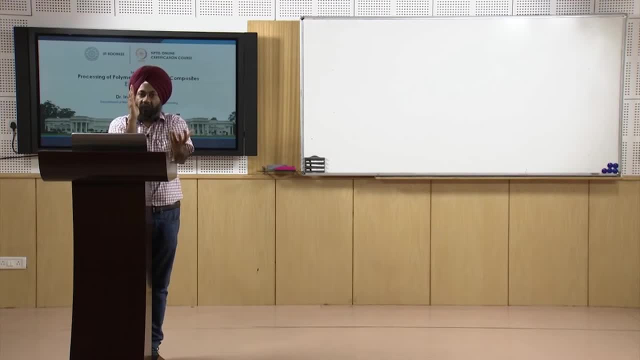 the, we can say, throat 16.. So the molten plastic enters into the barrel. then there is a rotating screw, there is a heating arrangement. The heating arrangement is heat providing heat to this plastic raw material. the material is getting melted. this melted material is pushed forward with the help of a rotating. 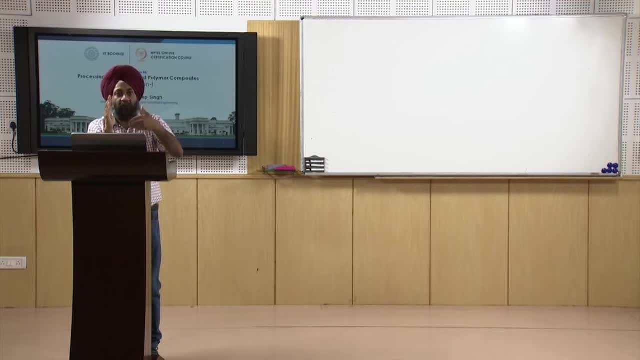 screw and this screw also results in the mixing and melting of the raw material. there is a screen pack which avoids the undue or the unwanted particles to move through, move along with the plastic, And then there is a breaker plate which provides the back pressure which ensures the proper 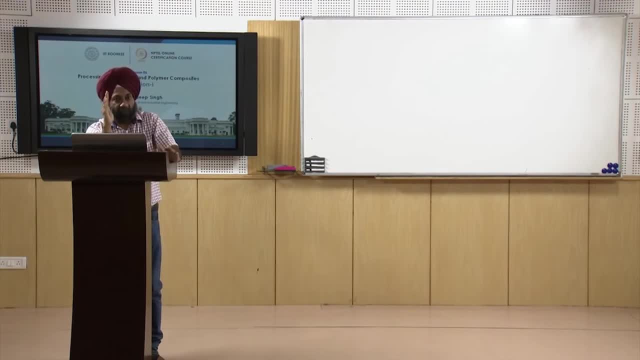 mixing and proper melting of the polymer pallets. So this thing has already happened. now the material is entering into the die and once the material enters into the die it will take the shape. So, as per our principles of processing of polymer, three things are very, very important. 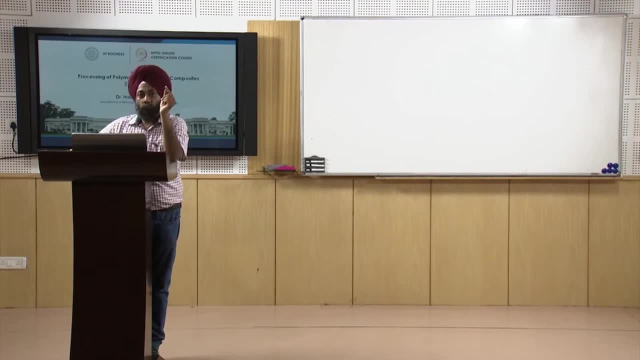 First thing is heating. we have to heat the raw material 17. So this is already happened till now. second is forming, that is giving shape to the raw material. So now the die will help us in the second step, that is giving shape to the raw material. 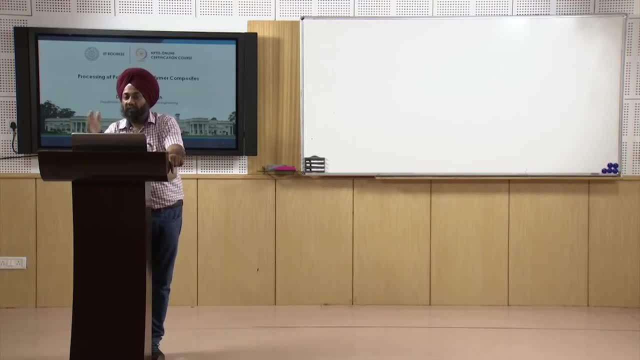 and third part is cooling. So cooling we will see later. now we have finished our stage one, that is, melting, mixing the raw material. Now the raw material is ready to be deformed into the desired shape, and that will be achieved by the help of a die. 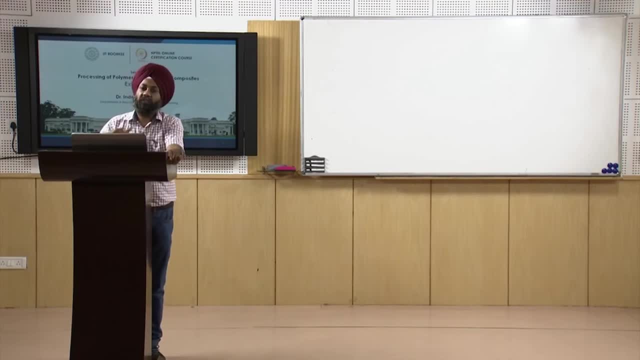 Now the after passing through the breaker plate 18.. Now we can see that the massa molten plastic is outside the die, so outside the biapper. I hold it for 10 minutes as to theory, as the roll is formed. ok, we have Vatc pequeña to. 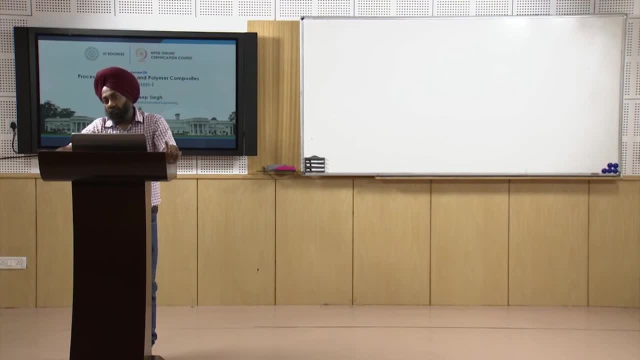 know that it is a pited solid. so the eraount aye of current, of current emmgentlement pressure, is known as em이션 higher stage. So we are getting to where is it doing that? 19.. has to be ensured now. plastics are very good thermal insulators. they are not good conductors. 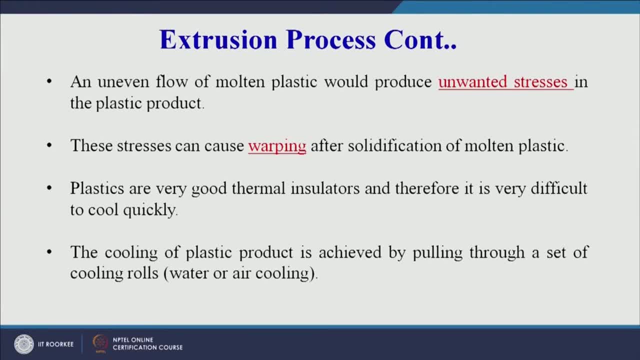 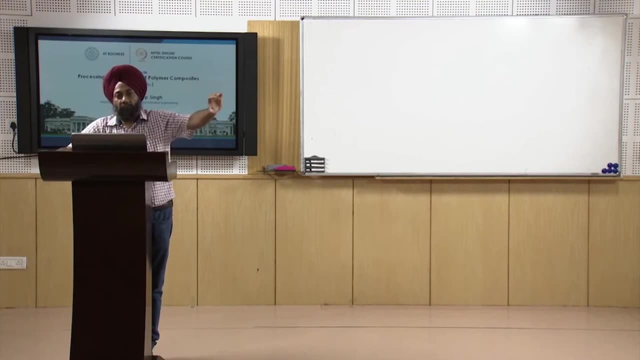 of heat and electricity and therefore it is very difficult to cool them quickly. so the cooling of the plastic product is achieved by pulling through a set of cooling rolls, as we have seen in our diagram, though we can always supply water cooling or air cooling for making of gardeners pipe or horse pipes. the product when it comes out from the die. 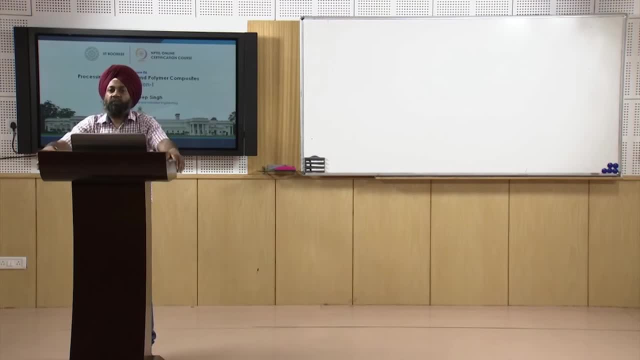 it is fed through the water. there is adequate length of this water column or a water chamber through which the product is passed, and when it comes out of the water chamber or water channel, it is solidified and it is in the final shape, or it is in the useful shape, or 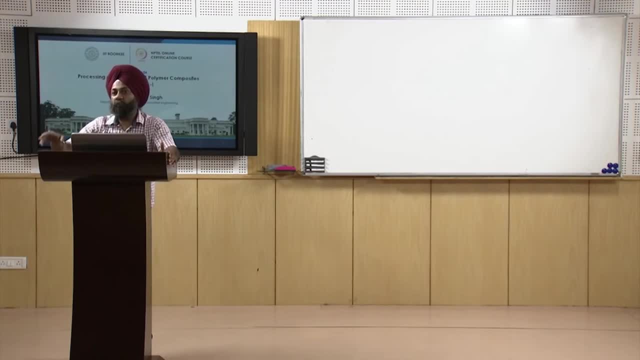 useful, it become the useful product. so cooling can be achieved through water also. cooling can be achieved through air also. so three steps now have been completed: heating, melting of the plastic, Deforming in the die and finally cooling, whether it is air cooling or it is water cooling. 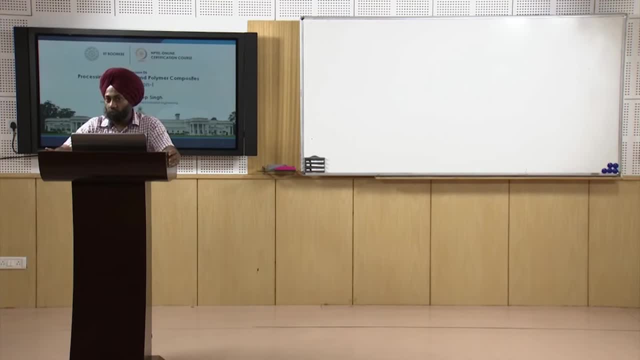 and on the way. there are two, three things that we have to ensure that no undue particles travel with the molten plastic. there is adequate mixing of the plastic and the additives that we have added. there is a uniform flow of the plastic through the die as well as after it. 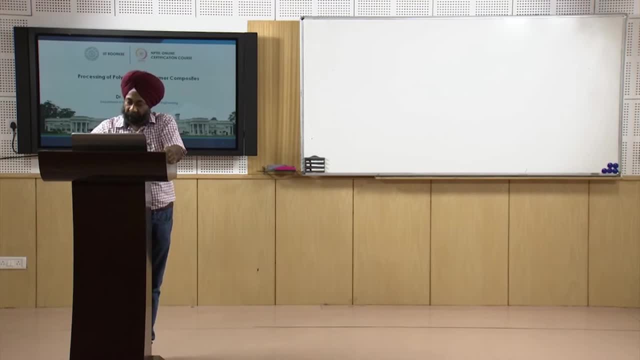 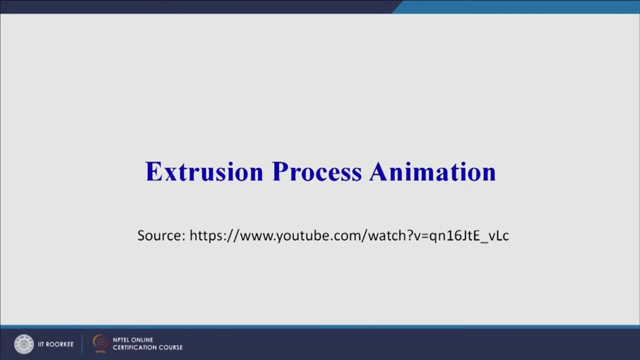 comes out of the die. that has to be ensured. now we will try to see a very simple, simple process In a verdian. Numbers of such animations are available on general platforms, general video platforms. one such platforms is YouTube. on YouTube, numbers of such animations are available as open source. 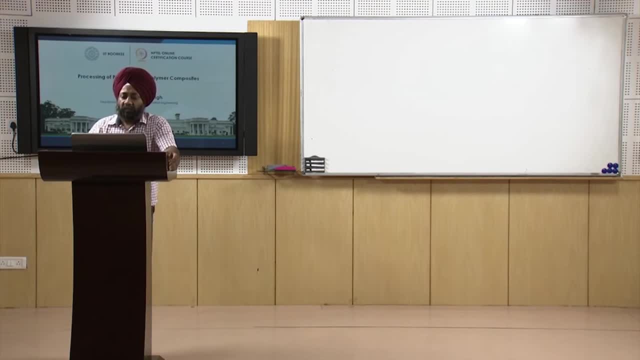 we have given the source, also wwwyoutubecom, and this video is available so you can see. there are other videos also available. for better understanding you can look at these videos Here. we can try to reduce the Investment Weulation. 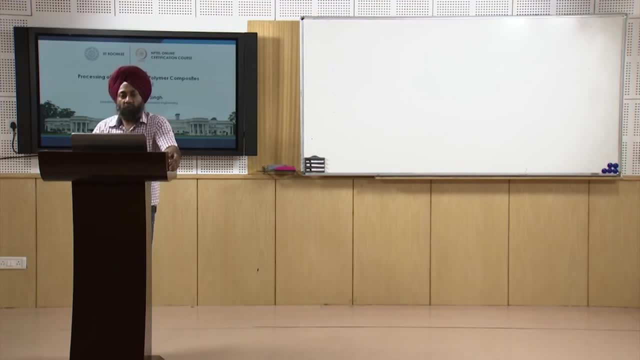 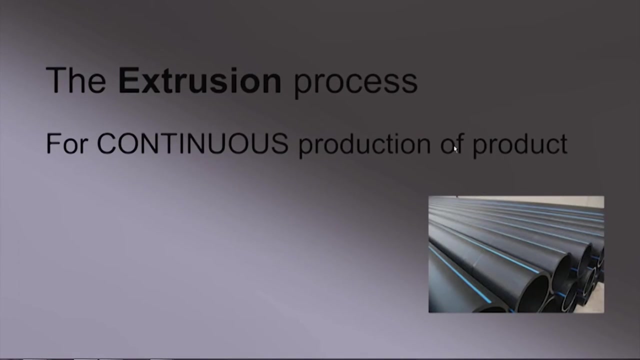 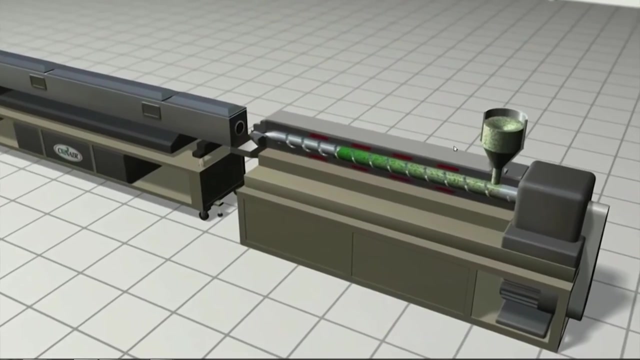 to understand how the process actually works. on your screen you can see this video. now the video is going to start and here also the it is mentioned. the extrusion process is a continuous process. here you can see the barrel is rotating, the material is entering through the feed throat, there is a hopper and you can see there is a coloring agent. 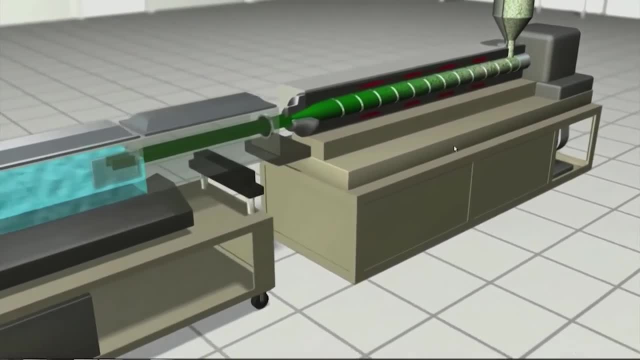 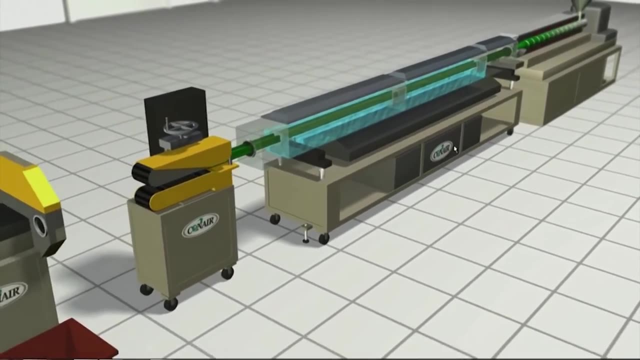 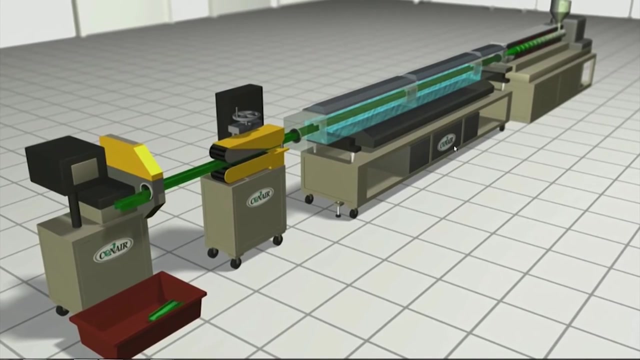 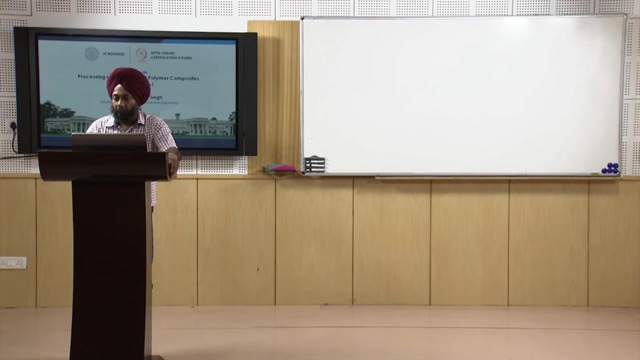 also plastics, pellets also, and the barrel is feeding it. then it goes into a water column chamber. it is getting cooled and finally the desired length. there are cooling rolls, then it is cut as per the desired length. you can see the products are falling down. so this is. you can see. you can try to understand. you can try to understand that. how fast is the? 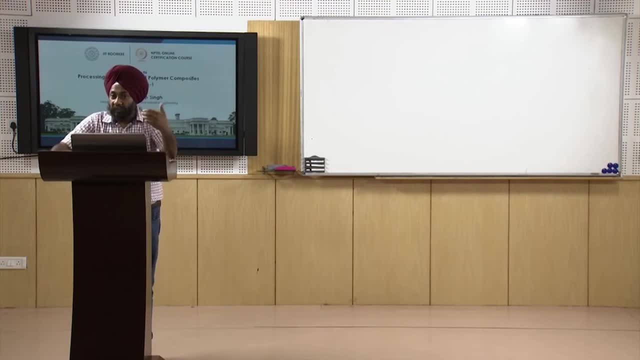 process. how continuous is the process. how time saving is the process? continuously, we have to feed the raw material in the hopper and once the hopper is full of material, the material will automatically, by gravity, go through the barrel as the rotating screw will rotate, and there 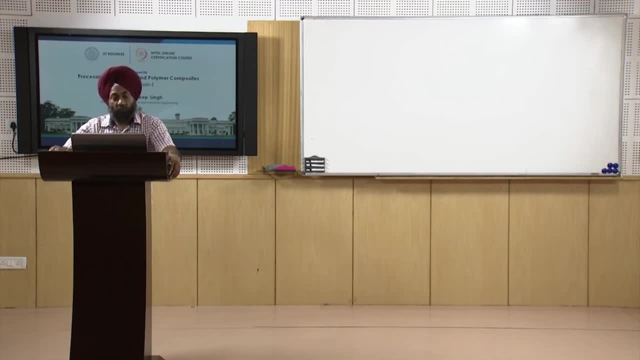 are heating arrangement. the molten plastic will be heated- sorry, the plastic will be heated- and then it will melt and once it melts it will travel through the die and it will take the desired shape. It will travel through the water column or a water chamber, it will cool down and, finally, 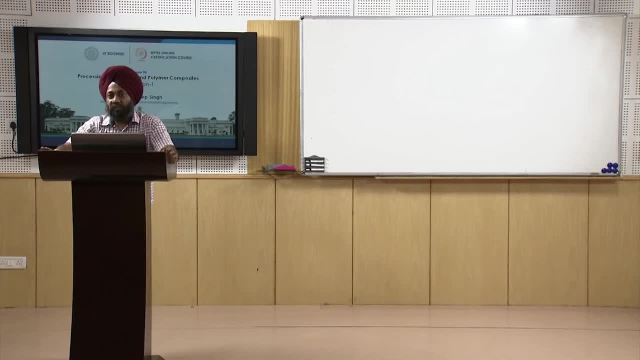 it will be cut as per the desired length. So the process, I think, is clear to each one of you if you have seen this video. Now, what are the parameters? as engineers, we need to design the whole process. we have to see that, what parameters we need to control and there are different types of polymers. 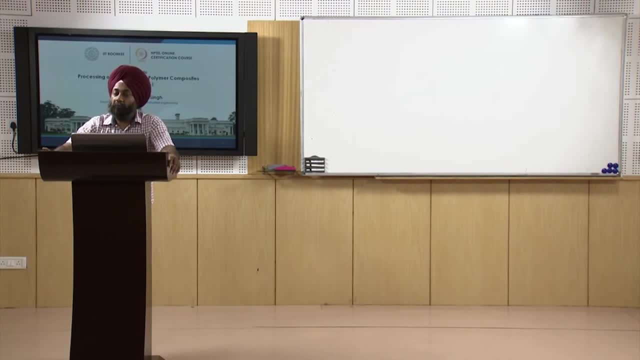 that can be processed by extrusion process. So, depending upon the type of the polymer, depending upon the shape of the product, depending upon the complexity of the shape of the product, we will see that what parameters we can control in order to make a good quality product. 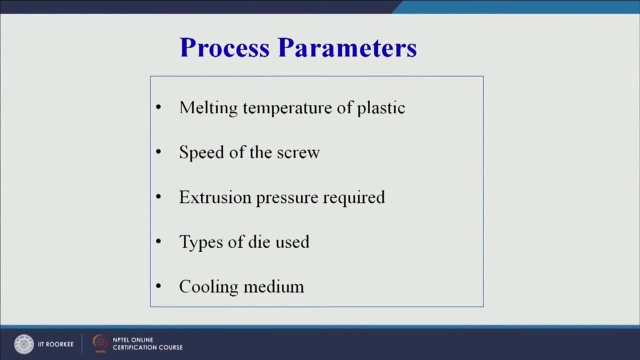 Now on your screen, you can see that we have different types of parameters that we can control. the first parameter that we can control is the melting temperature of a plastic. We have to see that, how, what heating arrangement we should use, what should be the temperature that we should generate. 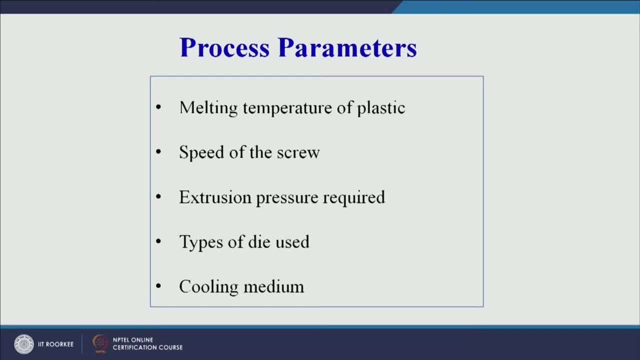 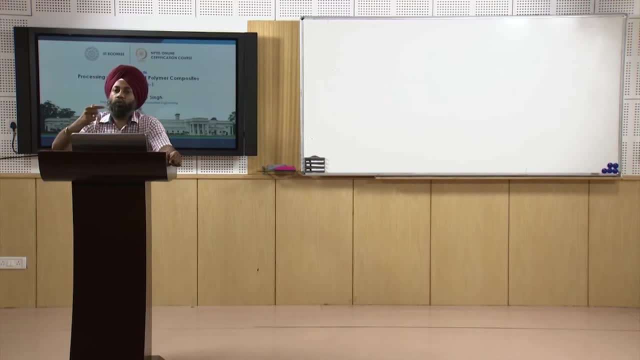 So that the plastic melts and it flows by the rotating screw. Second is the speed of the screw. you can see in this video the screw was rotating at a particular RPM. it can be increased also, it can be decreased also. So that will depend upon the viscosity of the molten plastic and depending upon that, 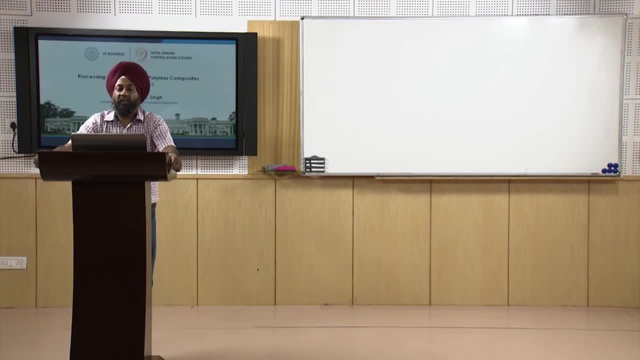 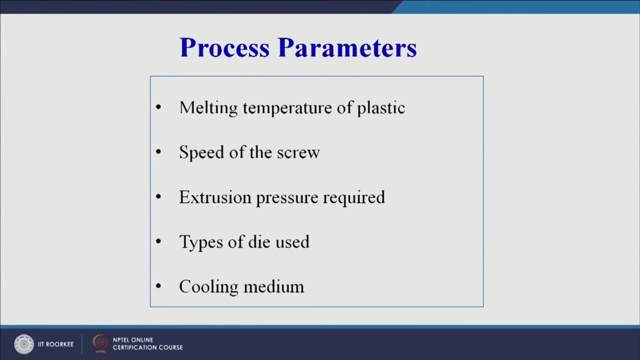 we will decide that what. at what speed the screw should rotate So that it melts the plastic also as well as it forces the plastic also through the die. Similarly, The extrusion pressure that is required. that will also depend on the RPM of the screw. 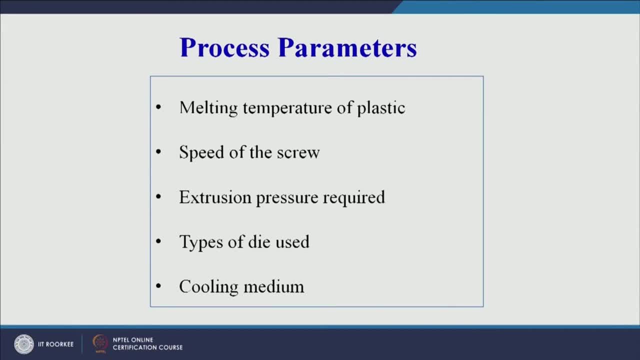 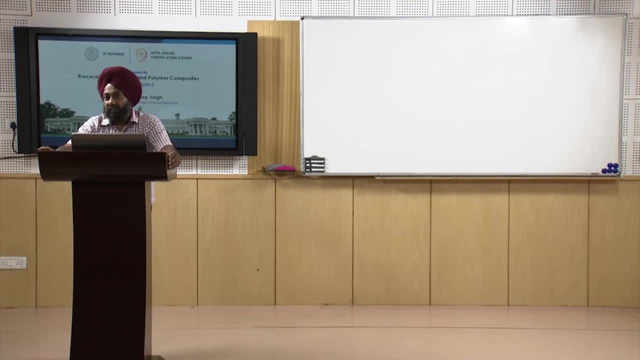 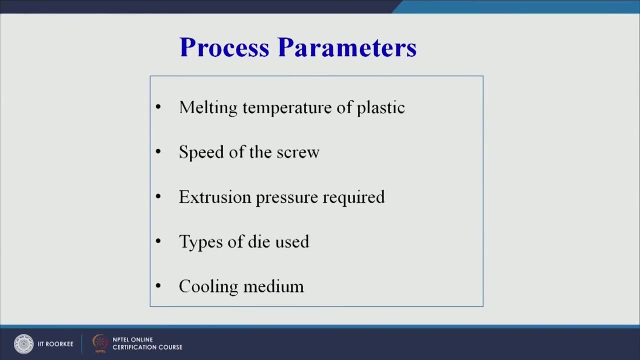 Similarly, the types of die used. there are number of types of dies which can be used which is beyond the scope of our this session, But we can see that the type of die that we select is also equally important. Similarly, cooling medium we have to see depending upon the type of plastic that we are using. 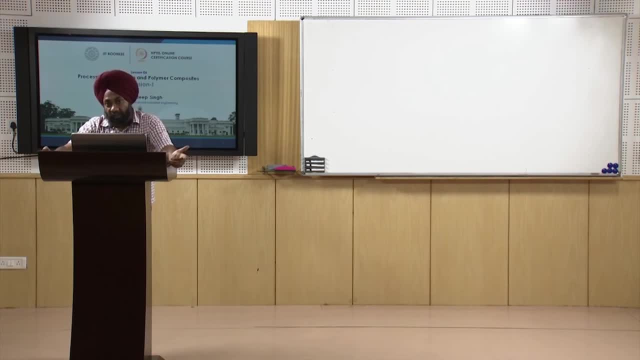 Now, cooling medium can be water, it can be air, It can be a jet of water, so, depending upon it, can be a column of water, it can be chamber of water, depending upon the requirement. we have to choose that what kind of cooling medium we have to employ. 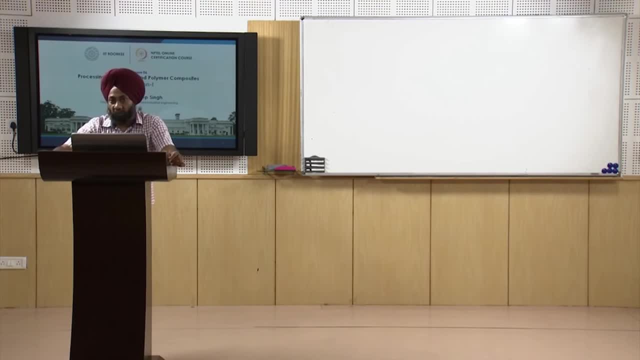 So that we get a good quality product. there are no defects in the product that we have to ensure. So these are the process parameters that an engineer has to keep in mind in order to design the process for a particular product. Now let us Come to the last part of our today's session, that is, the screw design. 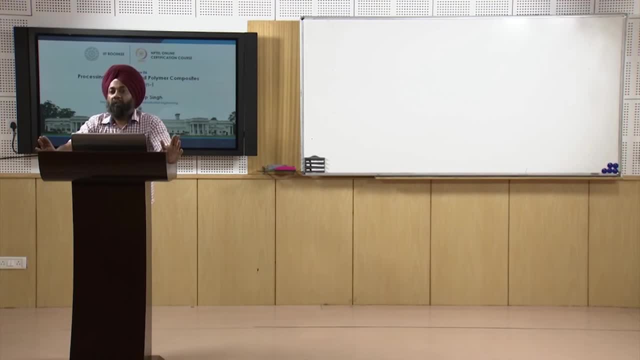 Now we see that we are. the major part of our process or setup is the screw as well as the die. Now, these are the two important elements. Now, die design is beyond the scope, but for extrusion process we can just have a look at the screw that what type of screw is used for extrusion process? 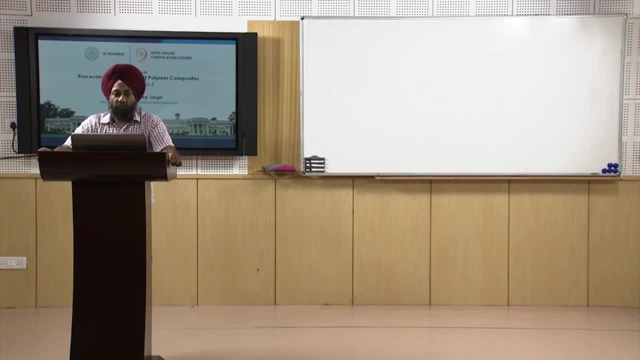 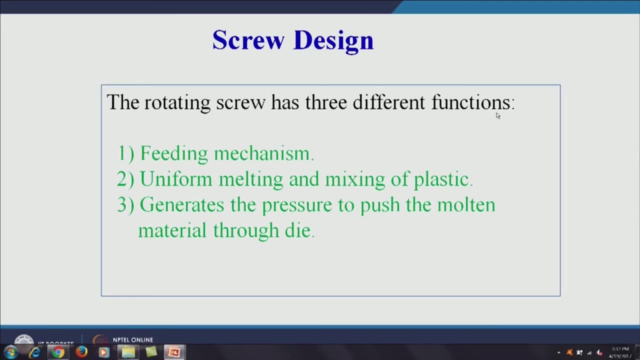 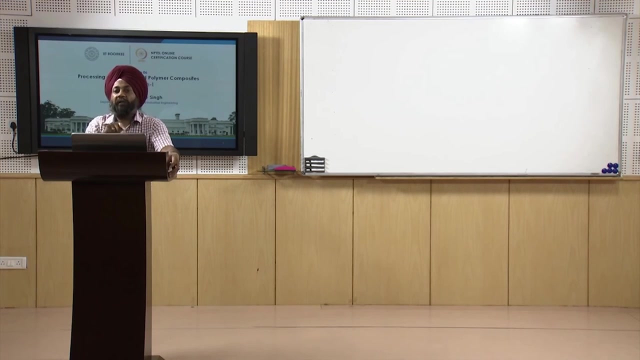 So the rotating screw has three important functions. First is feeding mechanism. If you remember the diagram that we have seen today, through the hopper, polymer pellets are coming down. Now these polymer pellets enter the barrel and then the screw rotates. So first is the feeding mechanism, that is, the screw is helping us in the feeding mechanism. 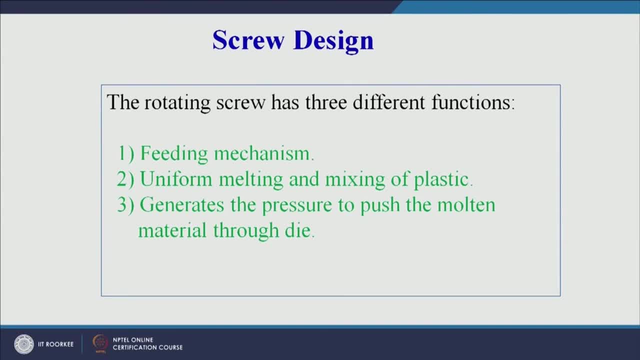 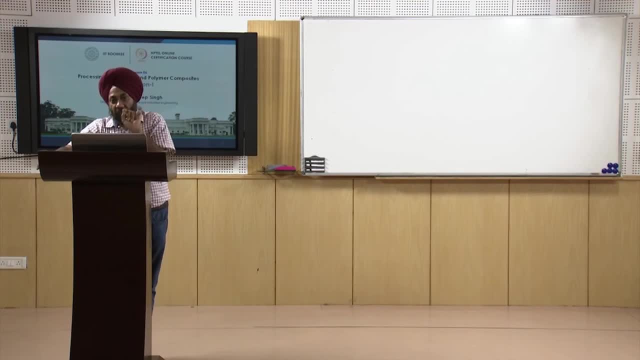 Second is uniform melting and mixing of the plastic. Third is it generates the pressure to push the molten material through the die. so feeding, mixing, melting And then pressurizing, that is, generates the pressure to put the molten material through the die or to push the molten material through the die. 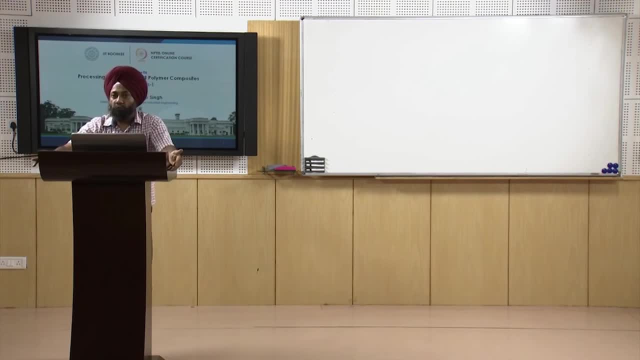 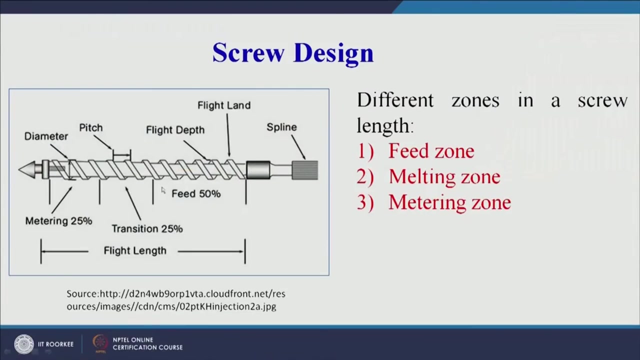 So these are three major functions of the rotating screw that is used in the extrusion process. Here you can see on your screen different zones in a screw length. So this is a typical screw that is used for the extrusion machine. There is a spline. 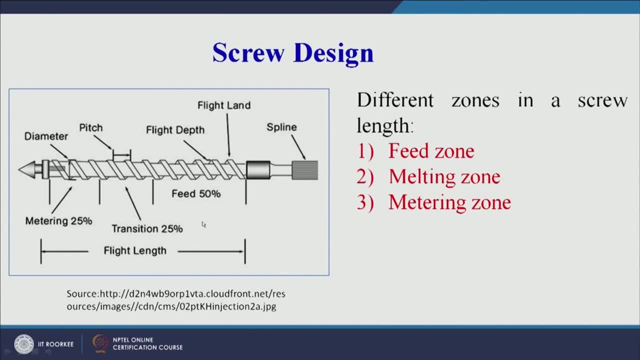 Then there is a flight length. Major part is these three zones. So there is a feed zone: 50% of the screw length may be usually is for feeding purpose. Then transition that we can say it is a melting zone. and finally the metering zone. 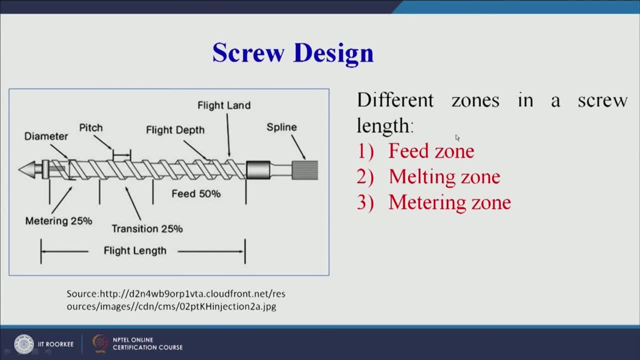 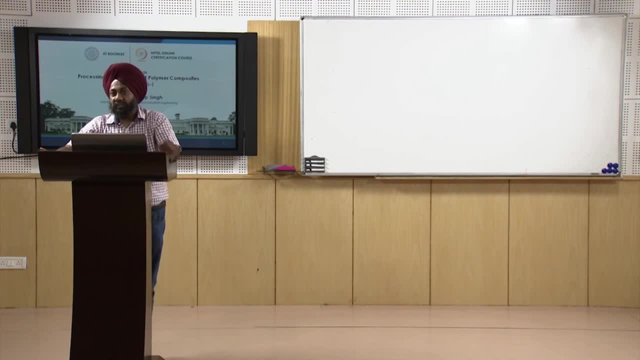 So basically different zones in a screw length are feed zone, melting zone and the metering zone. So this screw has to achieve three basic functions, that is, it has to feed, it has to ensure the mixing and melting, It has to ensure the third part, that is, pressurizing the molten plastic into the die. 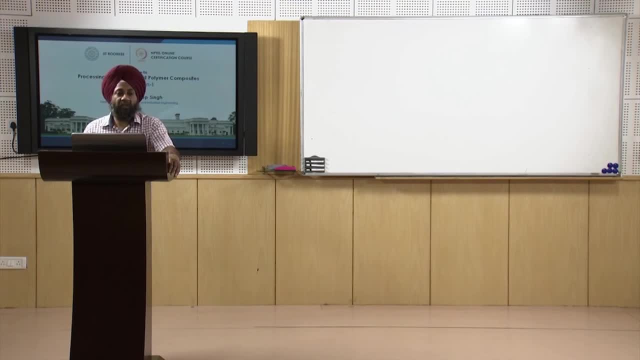 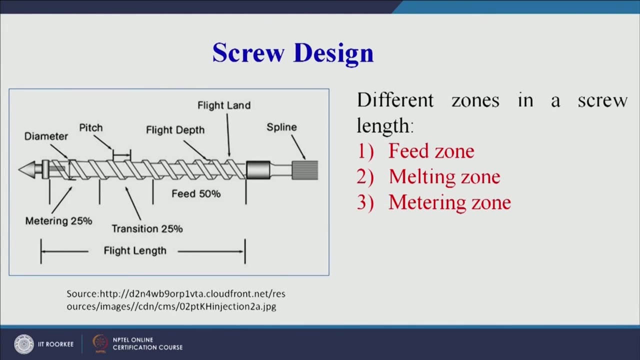 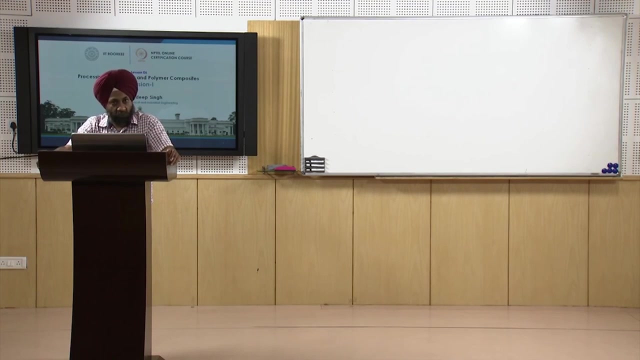 Therefore, there are three zones, basically feed zone, melting zone and the metering zone, to ensure that we get a good quality product. With this we come to the end of today's session. We have discussed today the fundamental process mechanism of extrusion process. 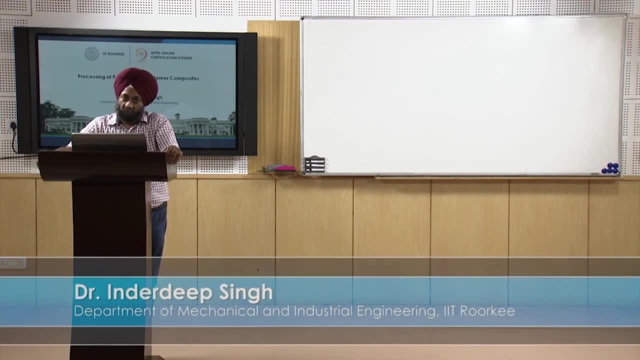 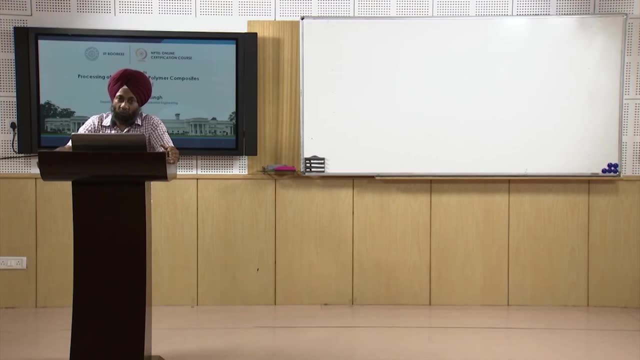 We have tried to understand it with the help of a video. also, We have seen That what are the various operating parameters that we need to control in order to make a good quality product, and in our subsequent session we will further see that what are the various types of extrusion processes or what are the process variants of extrusion.